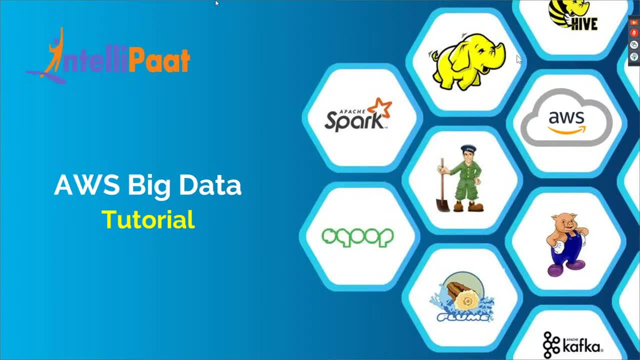 Thank you. Hey everyone, welcome to this live session by Intellipaat. So we're going to start off this session right now, So let me first explain what we'll be doing in this session. So first of all, this is an AWS Big Data. 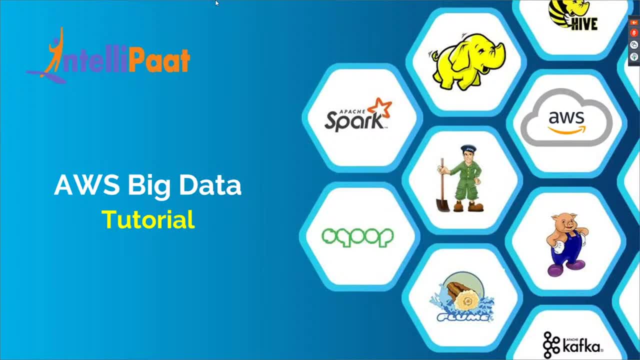 tutorial. So we'll be going through what is Big Data and also why Big Data on AWS. you'll have to choose, And then we'll be looking into the services which AWS provides for Big Data. Once that is done, we'll do a simple demo which will be on Hive, and we'll be hosting Hive on AWS, EMR, And the process we'll be doing is we'll be connecting EMR and on EMR we'll be having Hive and we'll be reading some data which is stored in S3. So that will do So. now let's move ahead with the session. First, let us 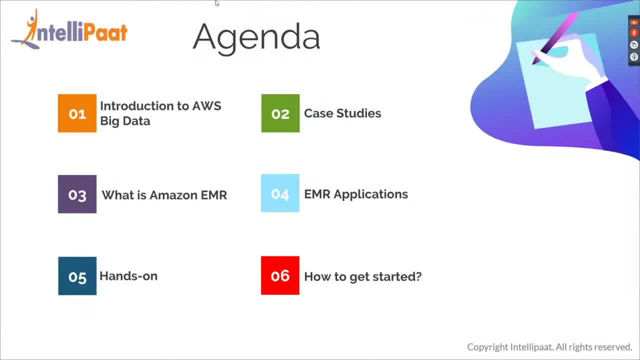 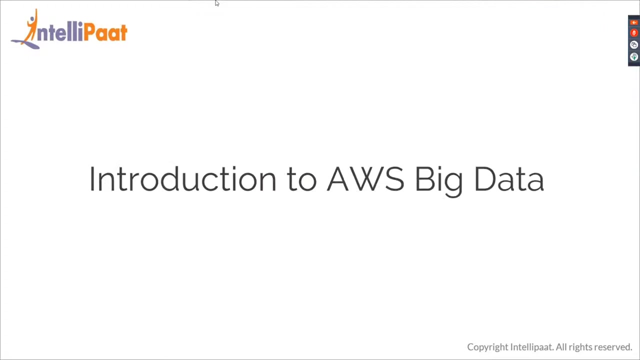 look at the agenda. Yeah. so first we'll start off with an introduction, Then we'll look into two case studies. Once that is done, we'll start off with EMR. I'll explain to you what is EMR in depth, And once that is done we'll do a quick hands on And finally I'll show you how to get started with your career or maybe your learning path. So first introduction to AWS, Big Data- Okay, so first of all, let's say Big Data analytics. 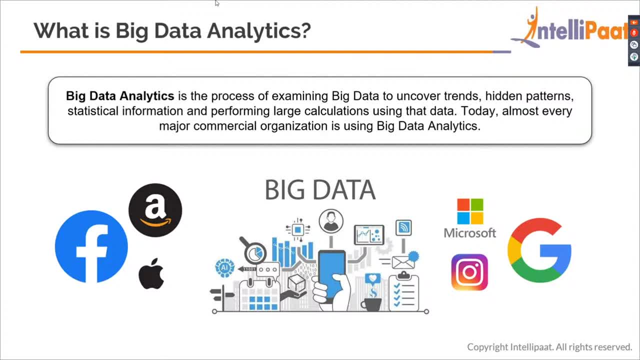 Because that's what we'll be doing once you have a large set of data. If you have a large set of data, the main objective is to get some meaningful data or meaningful trend out of it. So let's say there is a company and they want to grow, So what do they do is they'll be gathering a lot of data, maybe from the user end, maybe from the applications, And once that data is collected, they'll process that data. Once that data is processed, they will try to uncover some trends And they'll try to check some statistics, which 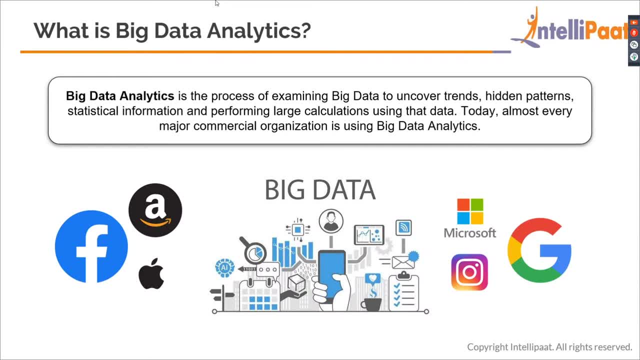 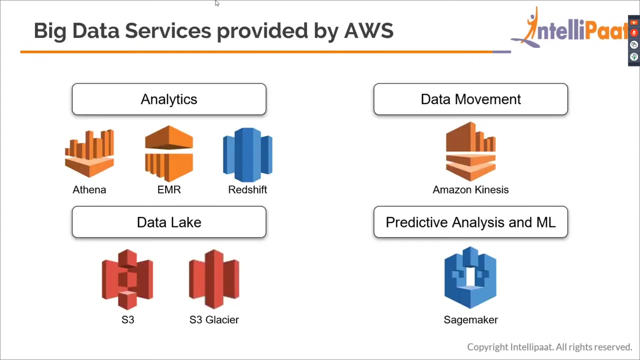 may be helpful for the business to grow. So you can see that today, almost every major commercial organization is using Big Data analytics. So if they obviously use, so these companies- Facebook, Amazon, Apple, Google, Instagram, Microsoft- so these all are major companies And obviously they'll be using Big Data, And so that's why Big Data is really important And Big Data is used everywhere. Okay, now we've seen what exactly is that, So it's simply. 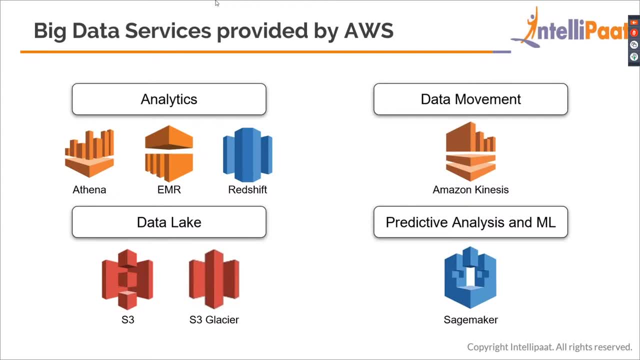 required. Okay, now we've seen what exactly is that, So it's simply required. Okay, now we've seen what exactly is that. So it's simply from a large set of data to get meaningful information is update analytics. So to do that, we have a lot of services, like in the local system we can upload, or on the on-premise setup we can configure using the hudu tools, using all the 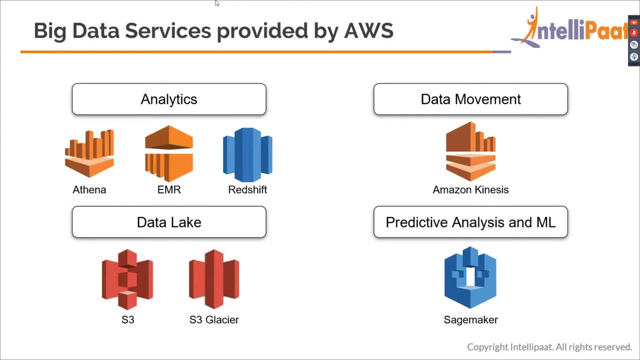 ah, duck, using all the, so instead, if you don't want to use that, you can use with the cloud. So again, in cloud that is Azure, there is GCP and also AWS hd ante, a customer of dcp and also AWS. So now, as we are looking into AWS, 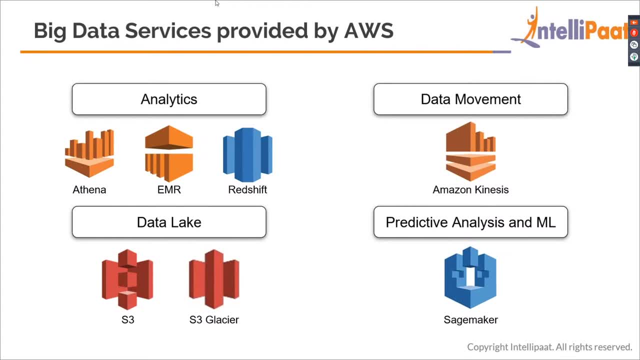 hosting, as we are looking into AWS. So I want to come back to you, But first we are going to talk about one of the other products. One of the other products we are looking into is… AWS. first let's look at the services provided by AWS. so there are four divisions in big data. 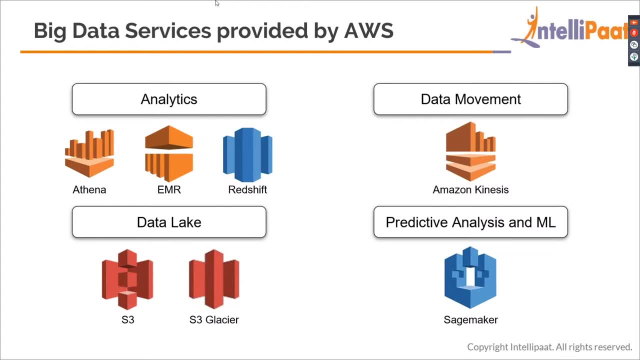 services provided by AWS. one is analytics, one is data movement, one is data lake and finally predictive analysis and machine learning. so first of all, in analytics, there is Athena, and then there is EMR, and then there is Redshift. so Athena is basically a query analysis software provided by 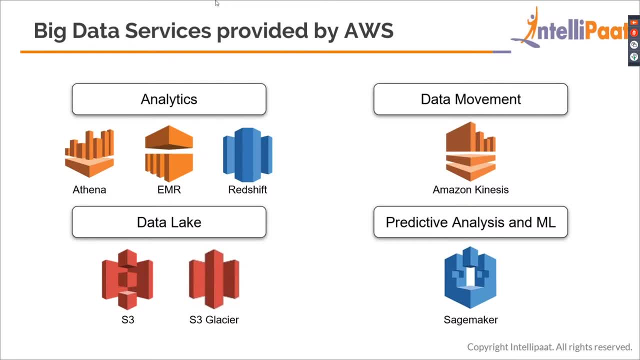 AWS. then comes elastic map reduce, which is basically a tool to provide the Hadoop ecosystem on a cloud level. and third, Redshift is a data warehousing tool. and then coming to data movement, this is for real-time data streaming. for example, if you are watching youtube, when you click on a 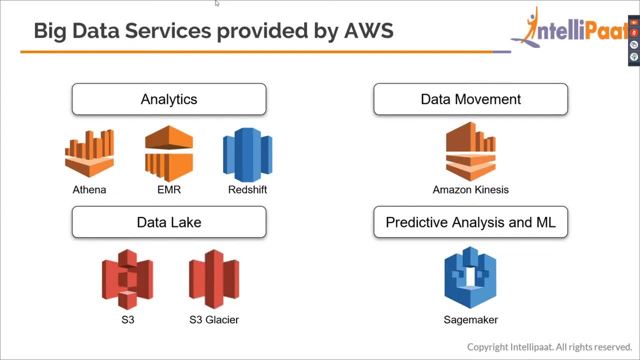 video. the video will be loading as well as you'll be watching the video. so, basically, the data is gathered from somewhere, and also your. you are able to access the same data at the same time. so for that you will be able to use Amazon Kinesis. and then comes data lake. so obviously to, let's say, to analyze data you. 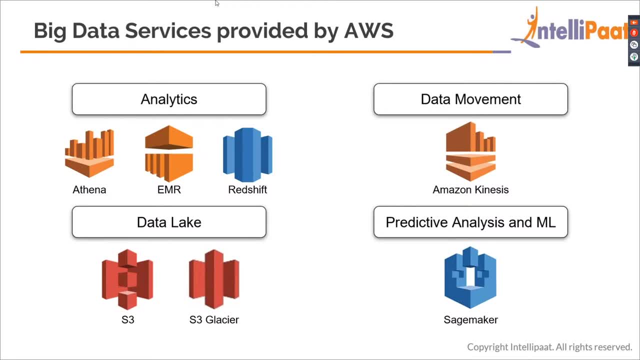 actually need to store data somewhere. so S3, and S3 glacier takes that part. so S3 is where you store your data. if you want to back up or archive your data, you can go with S3 glacier. and finally comes SageMaker. so SageMaker is an ML tool, so it's a machine. 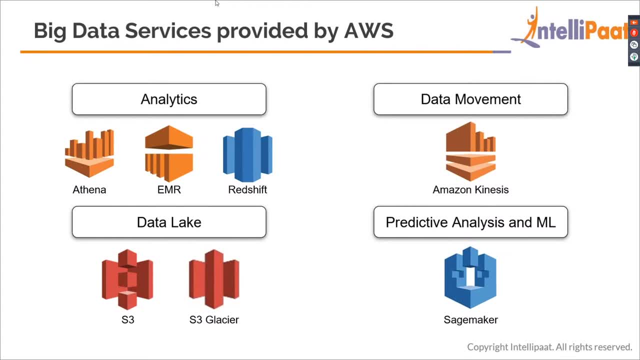 learning tool. if you know a little about AWS, there was a tool called Amazon Kinesis machine learning. currently it is deprecated and everyone are used moving to sage maker, because sage maker has all the built-in ml algorithms, for example k-means clustering. so if you want that, if you want to use that algorithm in your uh processing pipeline, then 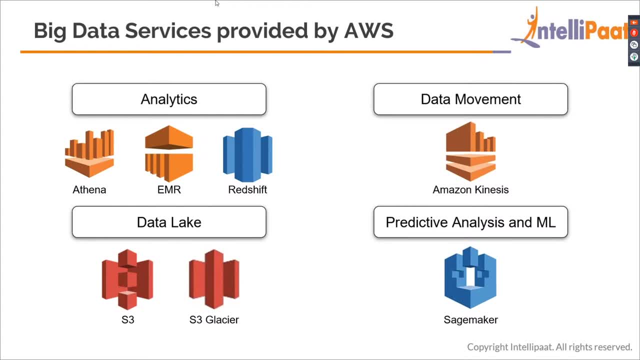 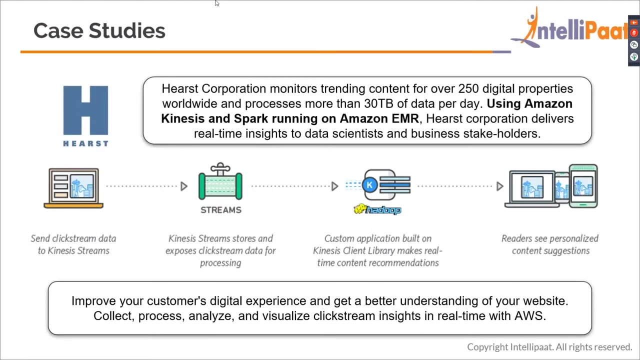 you can go with sage maker. it already has the built-in algorithm. you can just implement it. so these are the services provided by aws. so now, using these services, how do company get benefits out of it? so that's what we are going to discuss in our case studies. first of all, we'll be looking 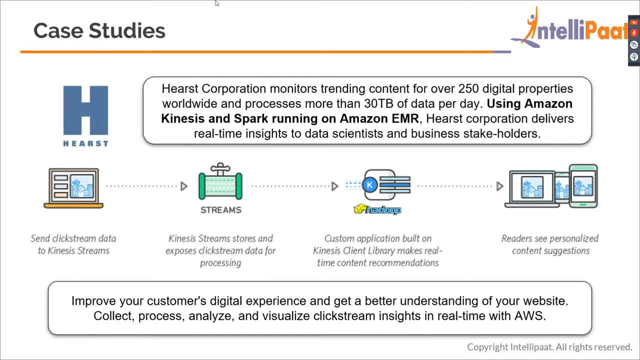 at two different companies: one is hearst and one is zillow. so you might not have heard of these companies, but hearst is a magazine company and zillow is basically an e-commerce firm who sell uh products. so coming to first. so hearst corporation monitors trending content for over. 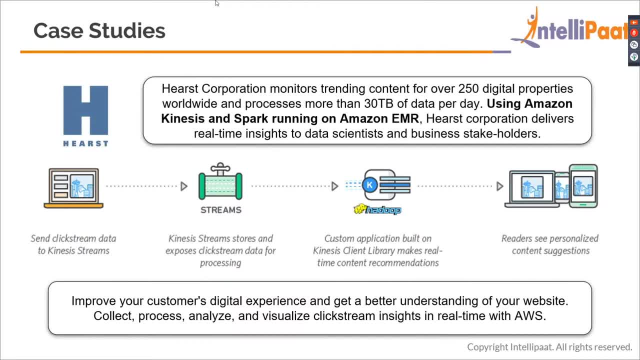 250 digital properties worldwide and processes more than 30 tb of data per day. so 30 terabytes of data per day is quite a huge amount and to handle that much of processing power you obviously need powerful systems. and therefore comes in amazon with kinesis to stream data, then spark running on emr to process data. so hearst corporation. 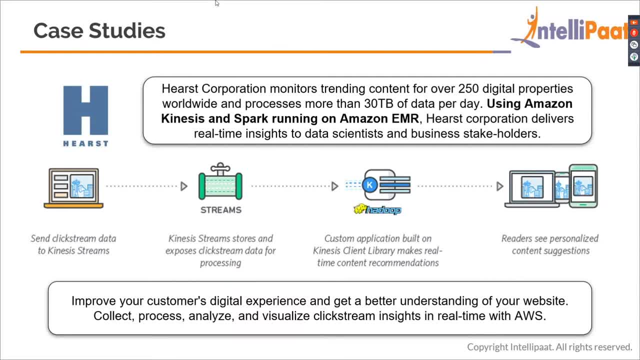 uses this to deliver real-time insights to data scientists as well as business stakeholders. so that's pure company part. so you can see the diagram in the uh below that. so first send clickstream data to kinesis streams, for example, if i'm a user, i'm reading a- uh, let's say i'm reading a blog on. 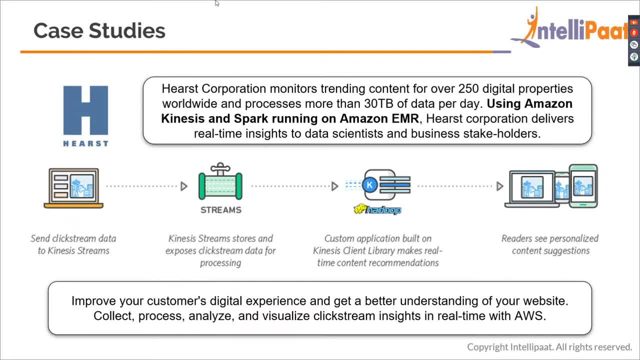 uh, sport, let's. let's say, i'm reading on a blog about cristiano ronaldo, so now, once i'm reading about that, so the next possible thing, uh, the algorithm should understand is that i'm interested in sports, i'm interested in football, so this person should be given football related content. 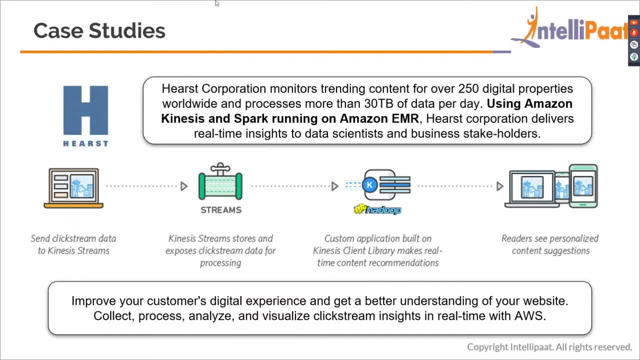 so that data will be taken. so kinesis takes all that data and it streams and it pushes into the uh client library which is running on the emr system. so on emr there is an spark uh spark system running, so you would have embedded your code in that so that processes the data and obviously 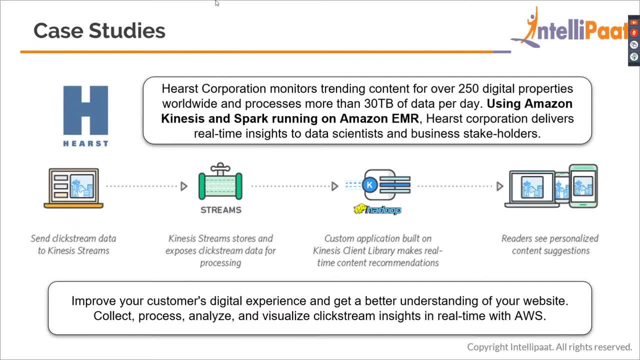 after that, the reader, which is i am- i'll be getting suggestions which are personalized. that is, if i'm reading about football, i'll be getting articles from other people and i'll be getting more and more articles related to football. so you can see at the bottom: improve your customers digital experience. 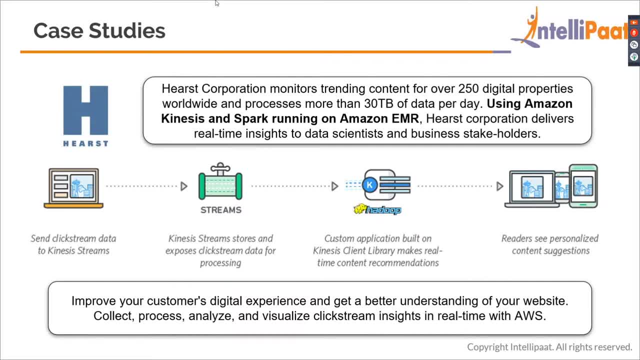 and get a better understanding of your website, collect, process, analyze and visualize clickstream insights in real time with aws. so to do this, you can see, you can use kinesis and spark. so that's what this organization is doing right now. so this is one of the one of the real-time case studies. 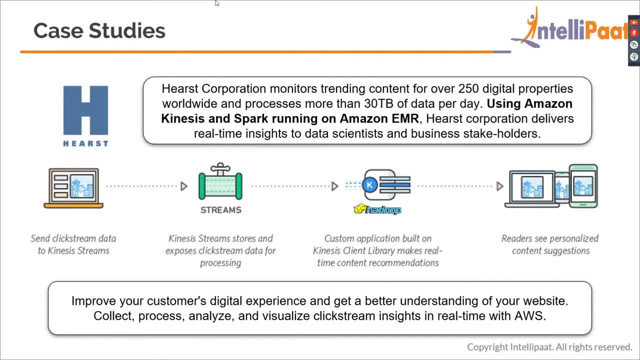 and i think you can understand this part- why. how exactly is big data on aws useful for them? one more benefit is that they don't even need to manage anything over here. everything will be managed by aws. you will just have to set it up. next case study is zillow, so as 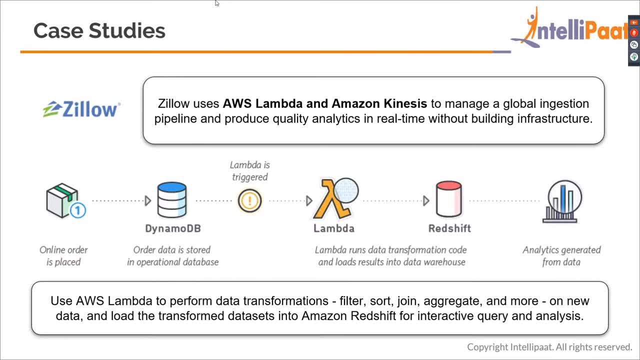 i told, zillow is a e-commerce platform, so zillow uses lambda and kinesis. so i didn't discuss about lambda, because lambda does not actually fall under the category of big data. lambda is basically a background. uh, let's say, to be more simpler, it's a software where you can put your code. 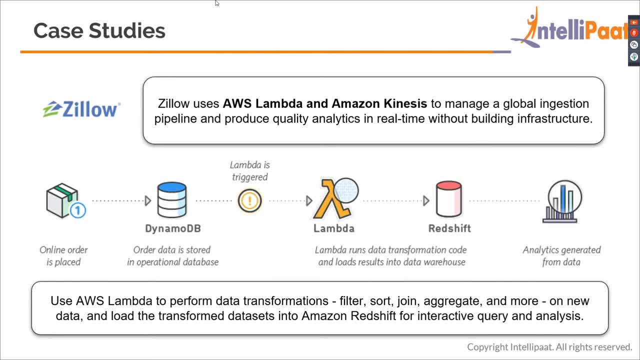 and whenever there is an event occurred. once that event occurred, this lambda function will be triggered and that code will run once. so this is why we use lambda, so let me explain that more clearly: so to manage a global ingestion pipeline and produce quality analytics in real time, without 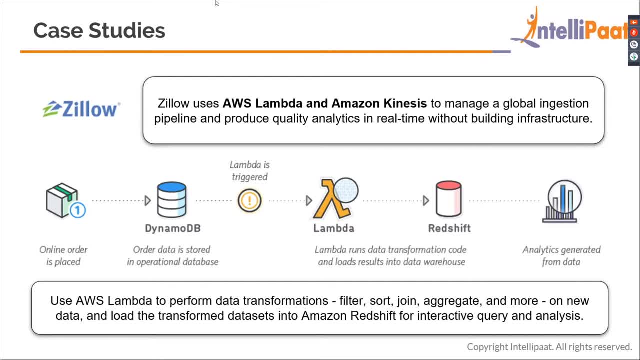 building infrastructure. so zillow is using aws because they don't want to build an on-premise setup. they don't want to build an infrastructure because that needs a lot of capital. instead they are opting aws. so first, uh. now coming to the diagram. so an order is placed, so i'm buying. let's say i'm buying a bottle. so 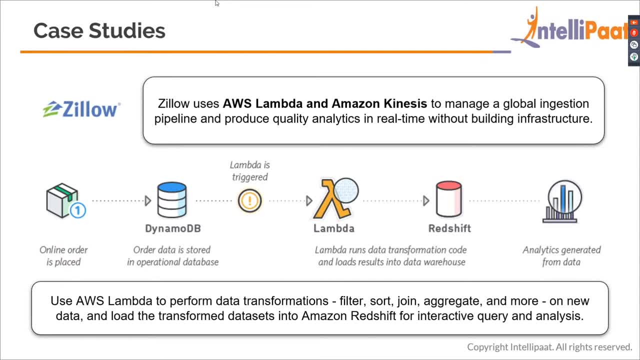 once i bought a bottle- that data obviously once the order is placed it will be stored in a database. so let's say that is dynamodb, so zillow is using dynamodb, so order data is stored in the operational database. so once that data is stored in dynamodb, so in lambda you have. 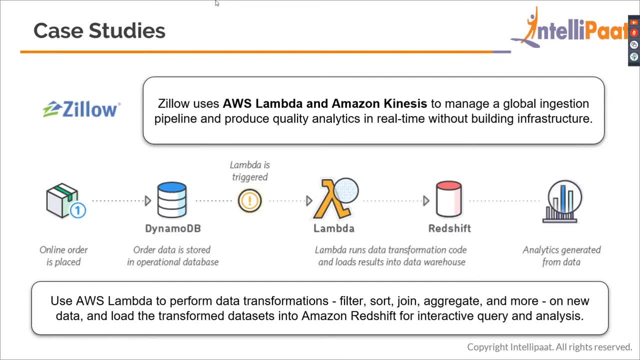 options to set up triggers. so let's say, in lambda our trigger is going to be: whenever data is getting into dynamodb, lambda should be triggered, and once it is triggered, the code in lambda will run. and once the code runs and the data is transformed, that data is pushed. 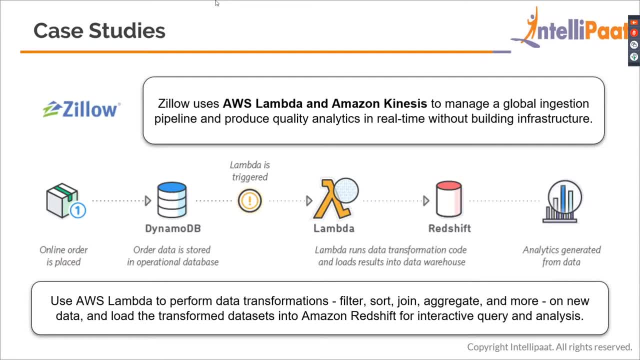 into redshift, which is the data warehouse which is mainly used for analytical processing, that is, to get data out of it and make visualizations and analysis from it. so for analysis you can use any tool of your kind: you can use power bi, you can use tablo, you can use amazon quick site, so you have a. 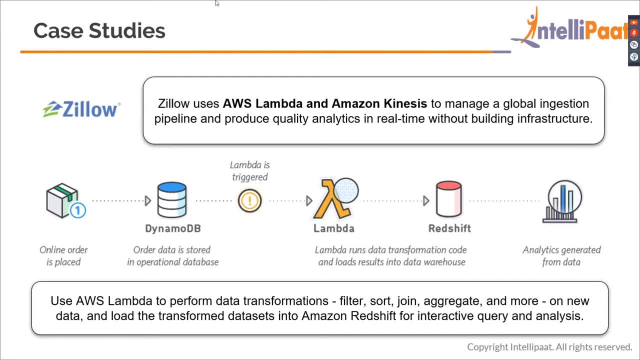 of possibilities, but the main part is you are storing data in dynamodb, which is a no sql database, comes lambda. whenever data is stored, lambda is triggered, lambda runs a code and that pushes the data into redshift, which is then used for visualizing data. so if you read the last para, 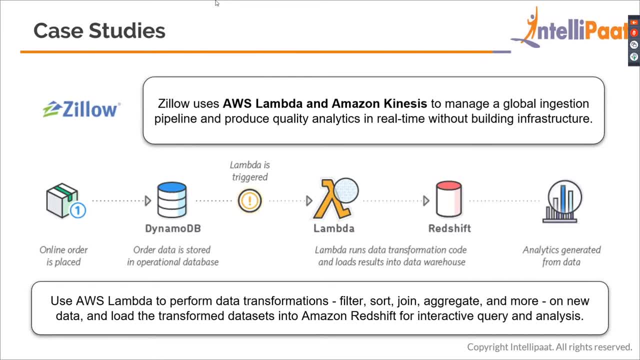 that is, use aws lambda to perform data transmissions- sorry, transformations- filter, sort, join, aggregate and more on new data and load the transform data sets into amazon redshift for interactive query analysis. so let's say, if you are uploading raw data to redshift, then there is there is no use for that because uploading raw data does not give you any uh ease of access. but 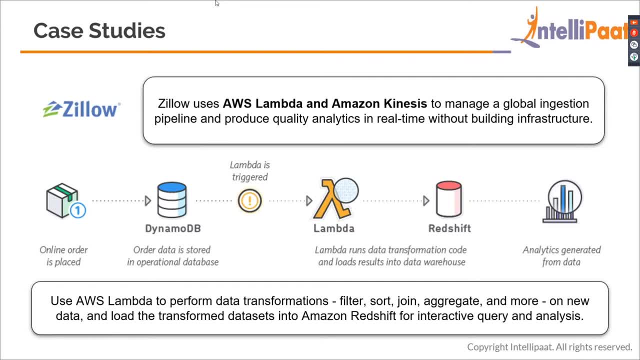 if you transform your data into easily readable format for the computer and easily queryable format, then if you push it into redshift it will be very easy for analytical processing. okay guys, just give me a minute. i'll just get some water. okay guys, i'm back. so we've seen the case studies. one was for uh hearst and one is for zillow. 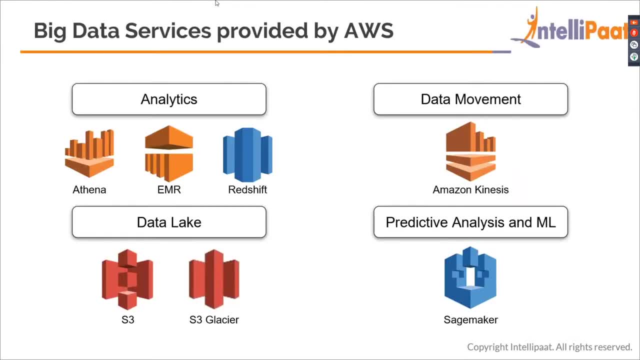 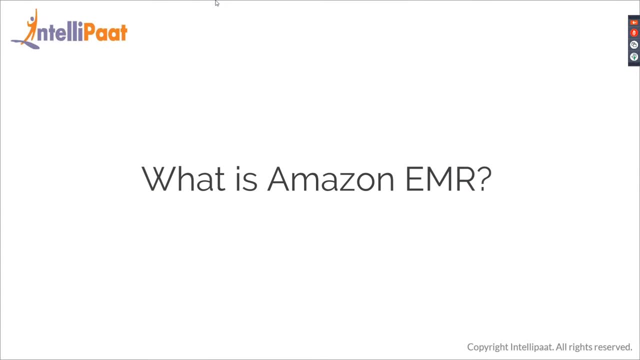 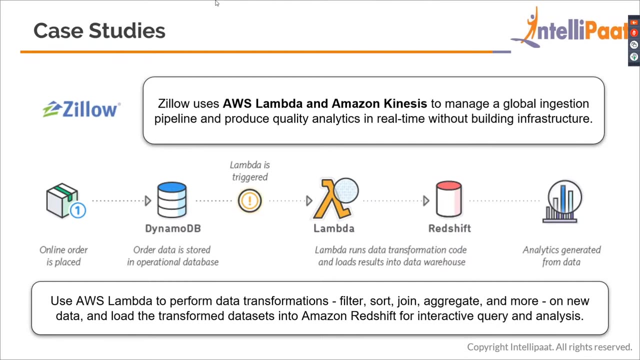 so we've seen that. we saw- yeah, we saw- about what is big data. then we saw the tools and we saw the case study. so one more thing why people prefer aws is there is no upfront cost. you only pay for what you are going to use. for example, if you are using a dynamo db for two hours, you'll only pay for. 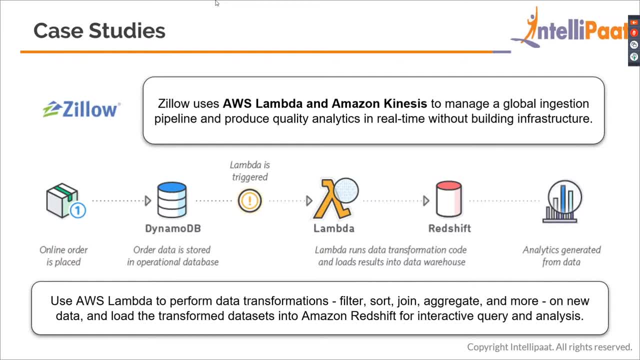 that two hours. also, it is very easy to manage you. it is scalable. that is, let's say, if you are currently having one table in your database and you are мал async, so you're going to need to purchase a table in your database and you'll only need to purchase. 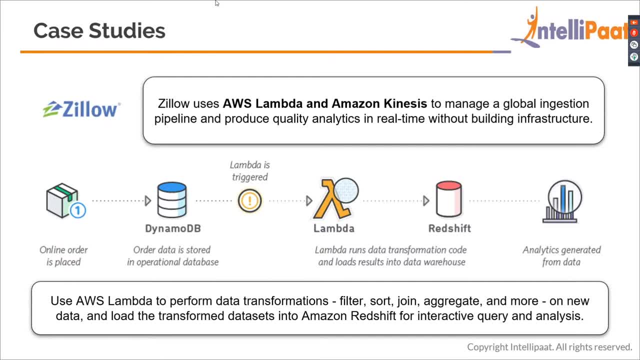 and you're currently having one table in your database with $100 momentum cost. so let's say, if you're currently having one table in your database and you're your database and it has 10 gb of storage, if you enable auto scaling if the data is incoming and 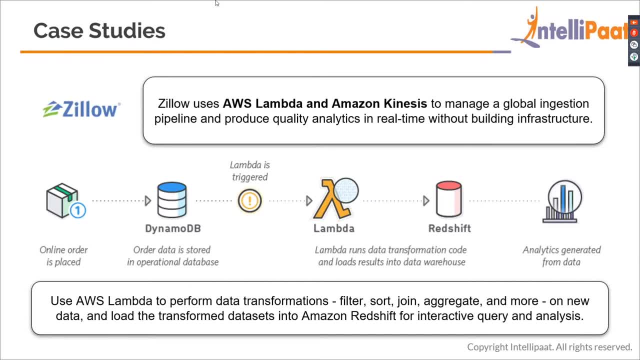 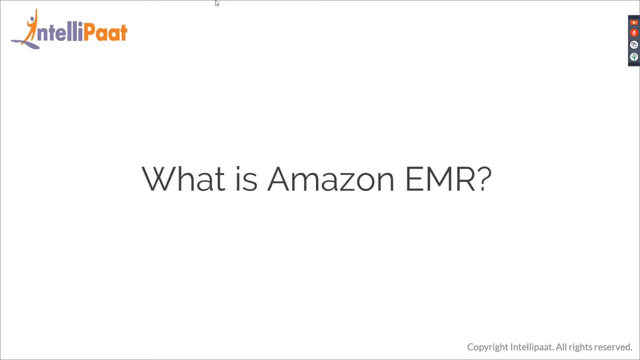 there is a lot of data to handle. it will automatically scale your database size to 20 gb and then increments, like, let's say, data is again coming in 30, 40, so it will be incrementing automatically. you don't need to worry about that. okay, so we saw that. now let's see what is amazon. 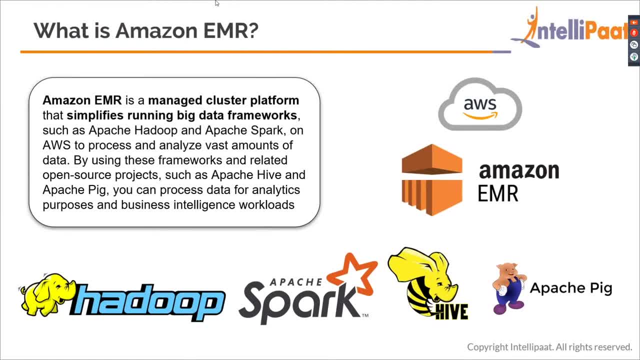 emr. okay, first of all, amazon emr is called elastic map reduce, so it is a managed cluster platform. that's sorry: managed cluster platform that simplifies running big data frameworks such as hadoop spark. so the thing is to understand this much more easily. i think you should have a little. 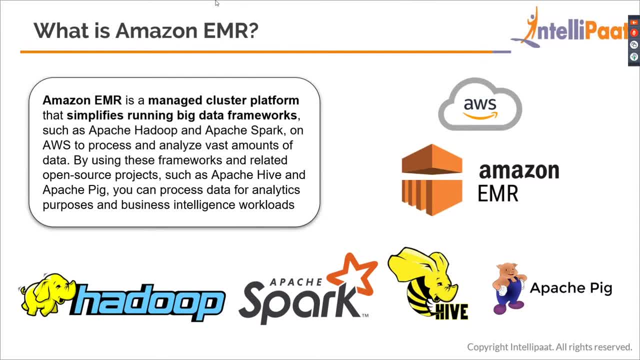 bit of idea about big data. so because there is no use of explaining uh, hadoop right now, because we are going to look at how, uh, these softwares for big data is used on aws, so just gather some little bit of idea. what is hadoop, what is spark? okay, so now on aws to process and analyze. 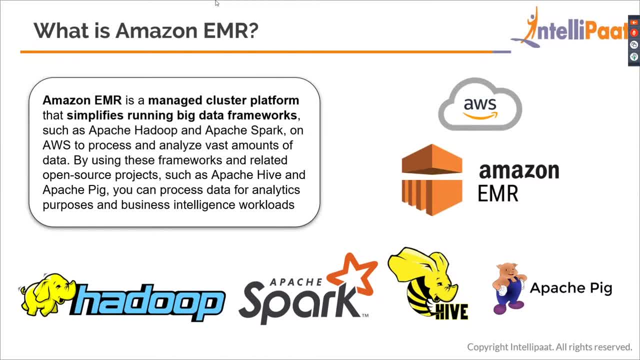 vast amounts of data. okay, so this is the purpose of emr: by using these frameworks and related open source projects such as apache, hive, apache pig, you can process data for analytics purposes and business intelligence workloads. so, first of all, emr is called elastic map reduce and it is a managed cluster platform. 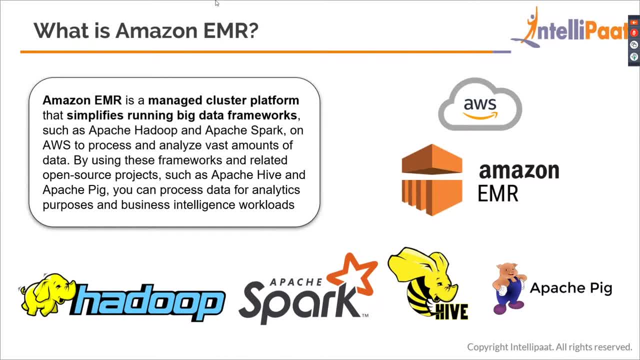 so this will simplify big data frameworks. so let's say you want to run hadoop on the cloud. so instead of running a server, downloading hadoop in that and configuring every single step, you can just go ahead with amazon emr. just type in the name of your cluster, choose the softwares. 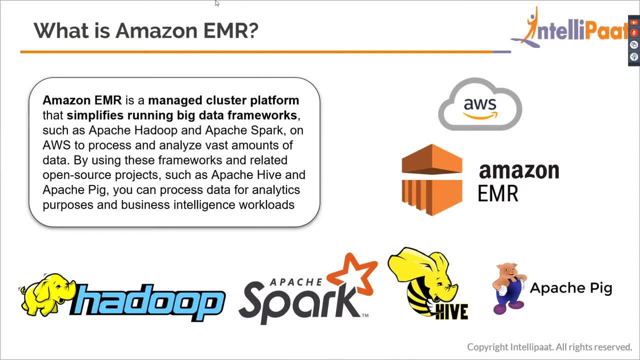 choose the big data tools which you need. once you've done that, you can give how many nodes you want. that's what i'm going to show you in a minute, so let's go ahead and see how that works. is the master and slaves? so let's say: one master, two slaves. you can have that once you mention that. 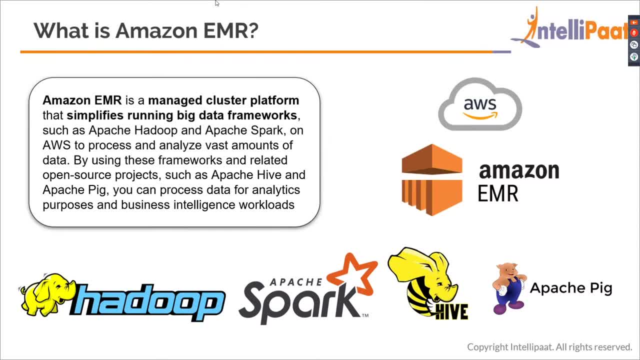 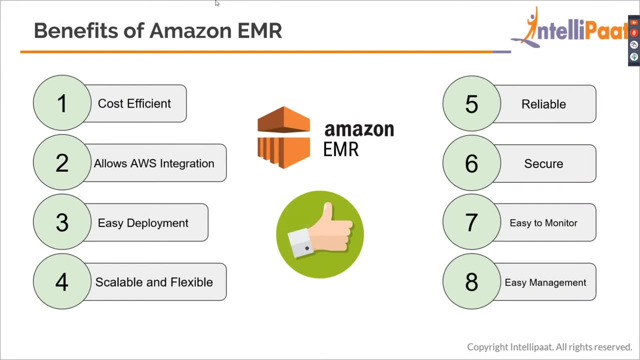 you'll have to provide a role and that's it. you'll just have to click on create cluster and it'll do the rest for you. so that's how simple amazon emr is. now let's look into the benefits of amazon emr. so, first of all, if you look into this, there is cost efficient, so that, as i told, you'll just have 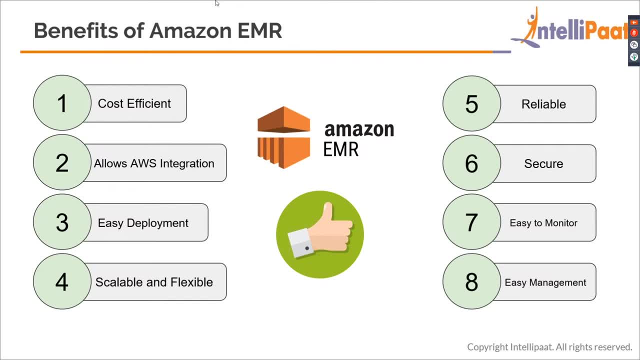 to pay as you go. then allows aws integration. you can integrate it with other aws services. then comes easy deployment. as i told you, you'll just have to give in few details and hit click. it'll automatically do that. and then come scalable and flexible. so, as i told you, there is auto scaling available and also it is flexible because you can terminate. 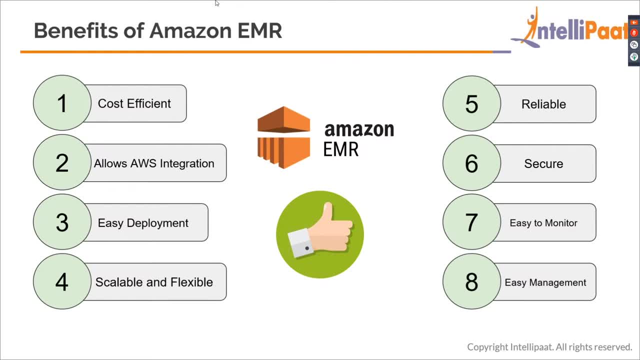 it. you can stop it whenever you want. it is reliable because they provide you an sla of 99.9, which basically means it never goes down. it is always on and then secure. so obviously it's about the same things, but the real value is the ability to apply the doc logo and then have a 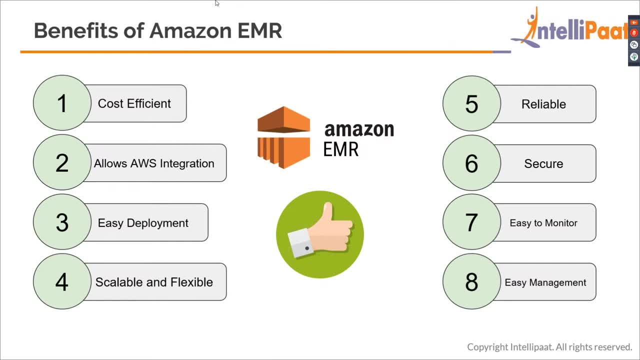 lot more features. so the next step i'm going to show you is using the aws server, which is basically like a web server, so you can use it as a web server. you can do that, by the way, with the aws server, which is an aws server, so it basically provides you a lot of security features. you can. 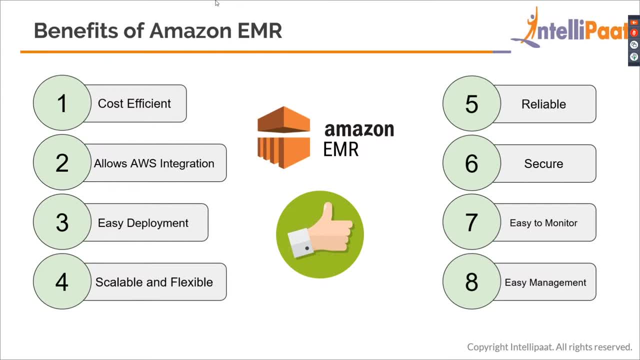 use iam, which is for identity and access management, where you give permissions to users, if they have. if they have the permission, they'll be able to use this particular service, emr. if they don't have the permissions, they'll not be able to use it, and then easy to monitor. so there is a service called cloudwatch. 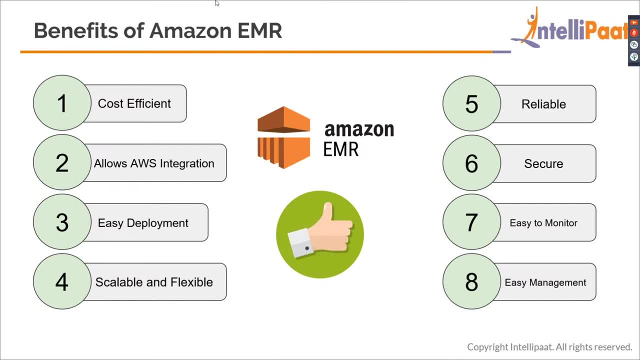 get the metrics automatically. finally, easy management. you're not going to manage anything, you're not going to patch anything, you're not going to add any code, you're not going to debug it. everything will be taken care by aws. you'll just have to set it up and that's it. so we've seen the 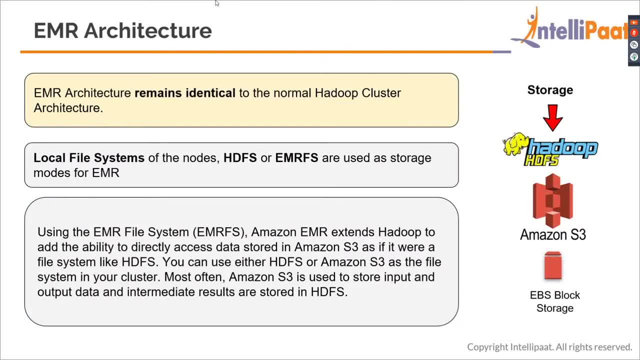 benefits, as well then the emr architecture. so how exactly it? uh, so how exactly it is, what is that hosted in the cloud? so that would be your question, right? so let's say, in your local system you would have the how to pick a system, because you'll know you will be downloading it, and then 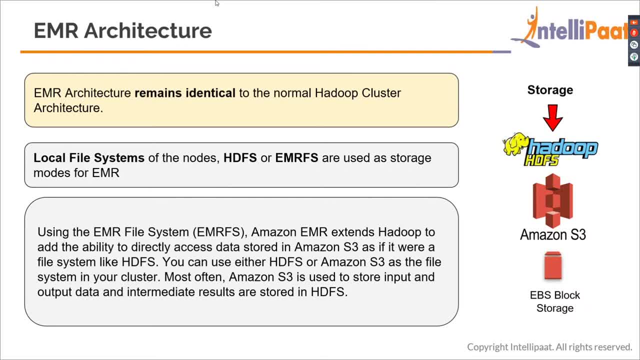 you will install it, you will configure it, you will set it up in the cloud. it is almost the same architecture, so you can see that emr architecture remains identical to the normal hadoop cluster architecture. local file systems of the nodes, hdfs or emrfs, are used as storage nodes for emr. so 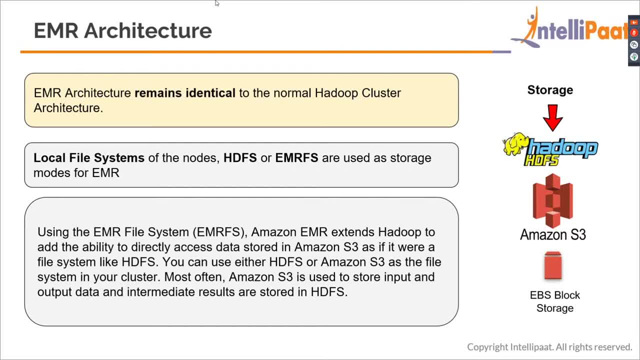 you can use the local file systems of the nodes, that is, local file systems in the sense the local file systems which is hosted in the cloud, so that local file system is basically amazon s3. so s3 is the back end for hdfs. so, as i told you, history is used for storage, so s3 is also used for storing hd. that is. 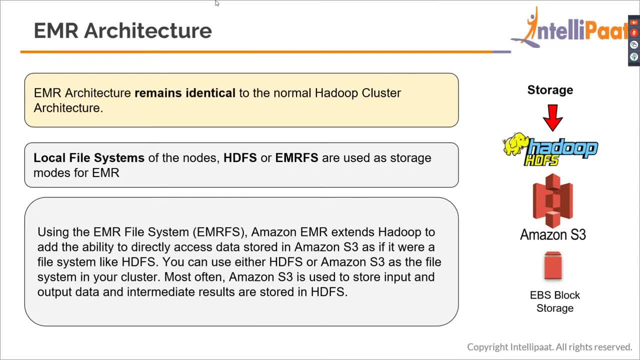 storing files in it. so using the emr file system, that is, emrfs. amazon emr extends hadoop to add the ability to directly access data stored in amazon s3. it is not that you will have to push the data into hdfs and then you'll you'll have to analyze it. instead, you can store the data in amazon s3 itself. 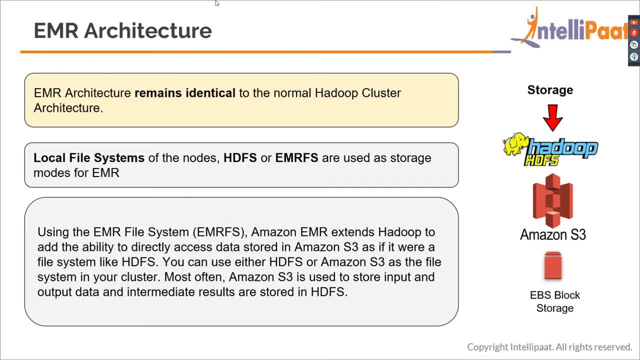 and directly from s3, sorry, yeah, so directly from s3, you will be able to query and analyze the data. most often, amazon s3 is used to store input and output data and also the results are stored in hdfs. so these are the temporary files are basically stored in hdfs: the input data and the output data, both. 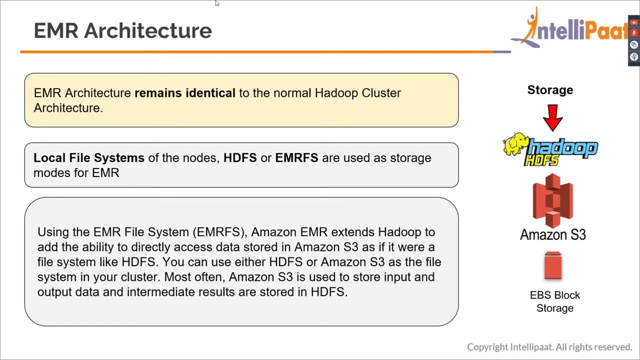 are stored in s3. so this is how it basically works, guys. it's pretty simple. it's a cluster format, or? uh? if you know about the big data services, it is the same architecture on aws as well. so if you don't know the architecture, i uh tell you. so i ask you to go, and please go. 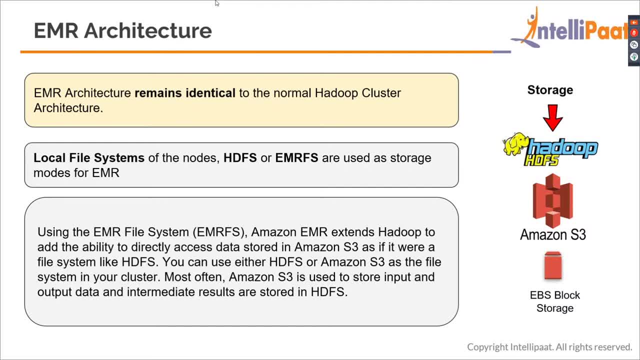 and check that out: check out hdfs, check out hadoop, check out map reduce and all that. so once you've get an idea of that, you will get an idea of how it is hosted on the cloud, because it's similar. so let's say it will have a back-end server running and in that back-end server hadoop will be. 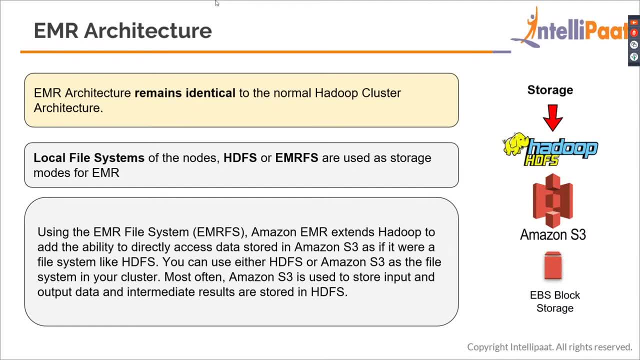 installed, configured and everything would be set up over there. and once that is set up, guys, amazon, s3, it is pretty simple. i'll show you how to start up with that as well, and then you will be able to set up, uh, whatever service you want: hive, hadoop, spark, uh, hbase, anything. 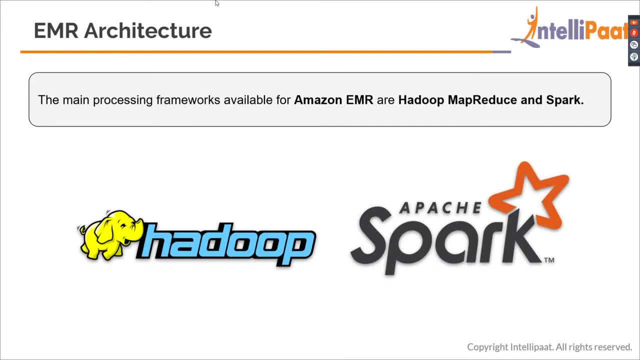 like that. so this is the basic architecture. okay, so the main processing frameworks available for emr is hadoop, map, reduce and spark. so one more thing: the, uh, most popular frameworks are hadoop and spark. there are other frameworks which you can use on emr as well, but the most popular ones 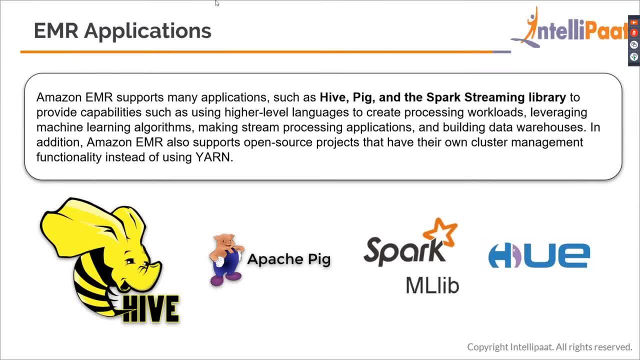 are hadoop and spark. okay, so now emr applications. that is, what are the other applications available on emr? as i told you, you can see over here, it's a box of all the products that has been introduced in the past and the ones that were. 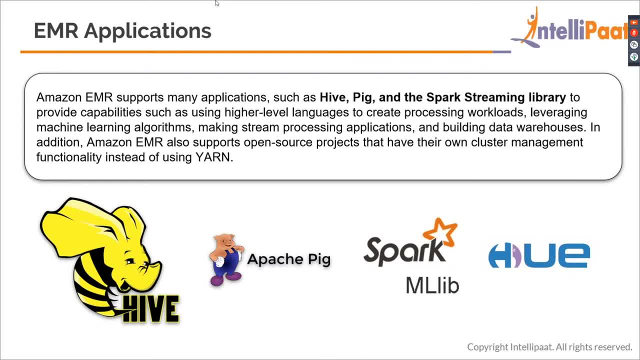 recently introduced, so you can see all these are uh. it supports many applications: hive pig, spark streaming platform. it supports yarn. it supports hue. it supports mostly all the uh apache products, that is, the hadoop ecosystem products, so you can go ahead and look into that uh more so we'll not. 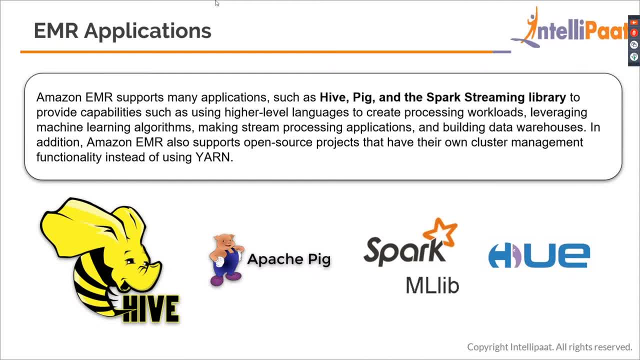 be covering this a lot now. next i'll be doing a hands-on using hive on emr, so let's do that. so in have their own cluster management functionality instead of using yarn. so, instead of using yarn, if you are using your own resource management, then that is also fine, so emr allows that as well. 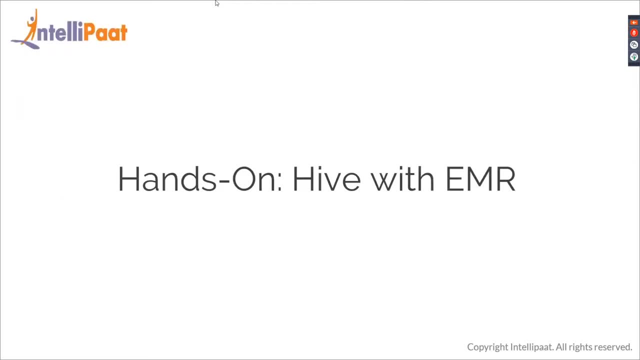 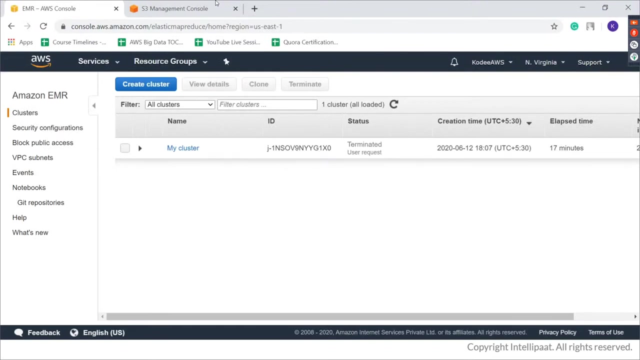 okay, guys, so we've seen that, so now let's do an hands-on on amazon. so this is basically getting to know session. so you will get to know how to start off with aws and aws big data. so first of all, to start off with this, you will need an aws account, so i suggest you to get an aws account. 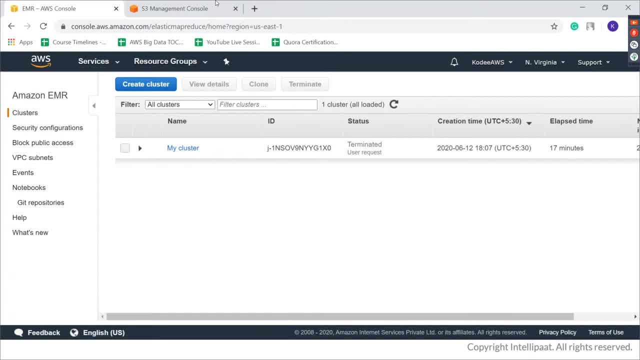 soon and start practicing, because this session will be available in our youtube channel and you can go through over that. okay, so right now i'm already in the emr console. i have logged in and it's pretty simple and you can just search emr over here and click here and you'll be inside the 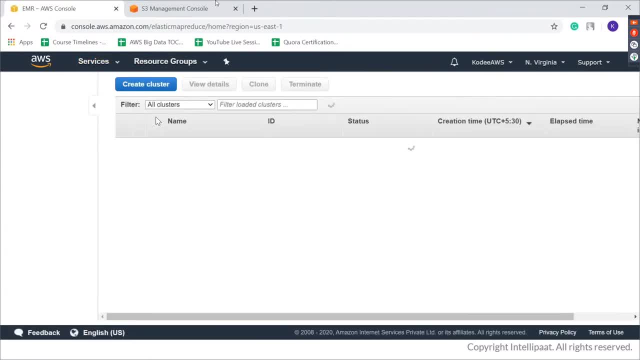 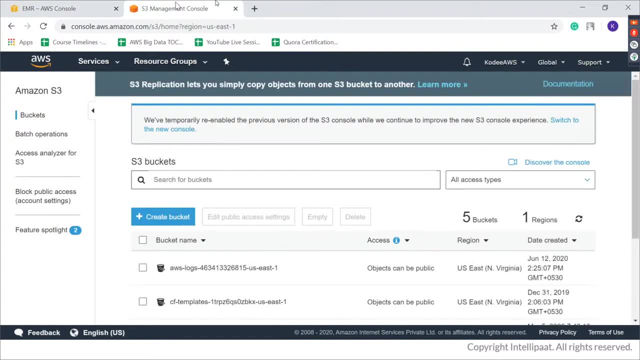 emr. yeah, so i'm here. so just one second. i'll have to show you s3. okay, first of all, let's uh create a bucket here. so what we are going to do, we are going to create a bucket to get our output, so our output will be stored in. 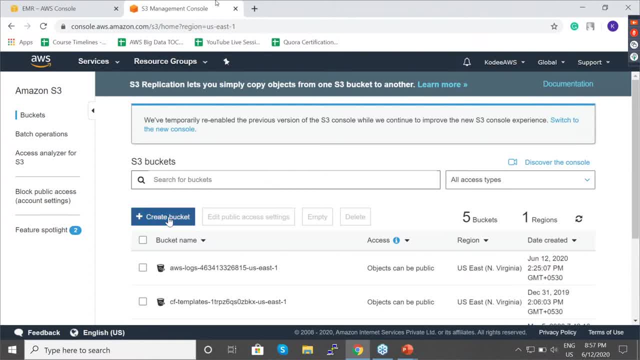 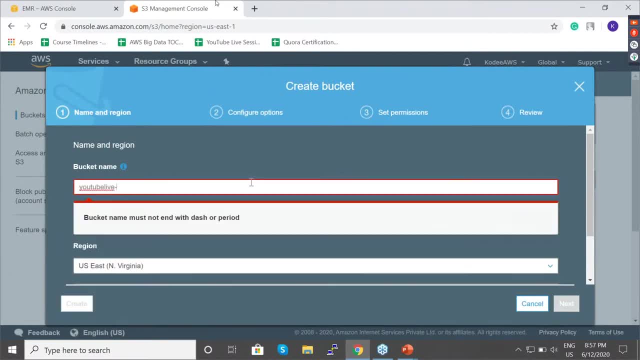 the bucket we are going to create. so this is the. this is very simple. click on create bucket, provide a name. so let me give as youtube live webinar one and i'm going to just create. i'm not going to set up anything, i'm just going to create a bucket and i'm going to create a bucket. 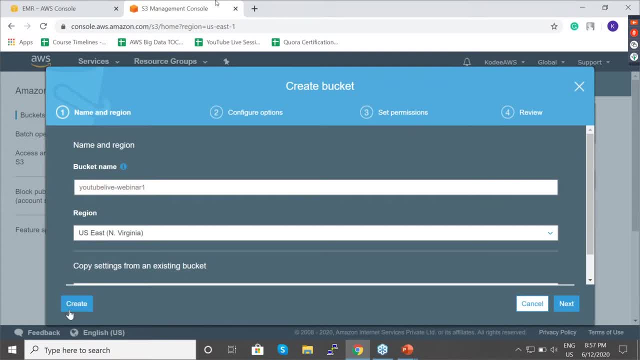 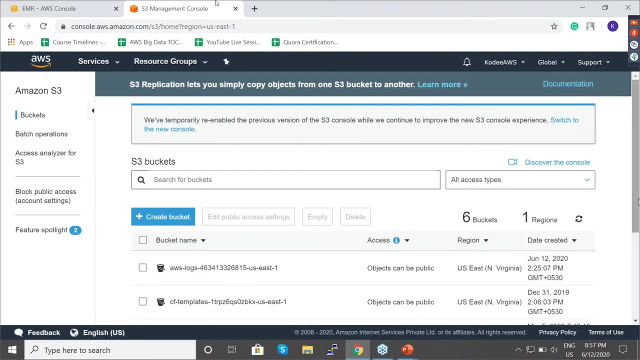 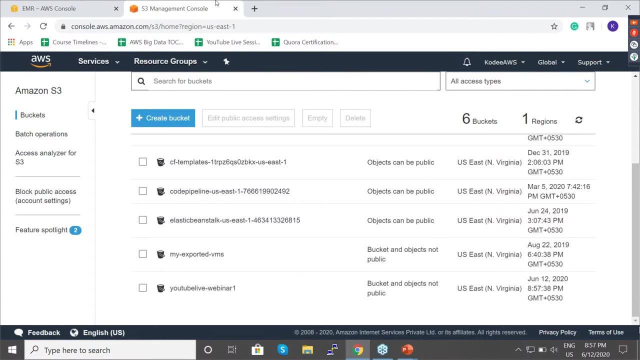 thing. i'm just going to create this. so it is this simple start bucket. so a bucket is basically a repository or a folder where all the files are stored. so it's pretty simple, guys. you just have to remember that. so a bucket is basically a folder where you can store all kinds of files. it may be. 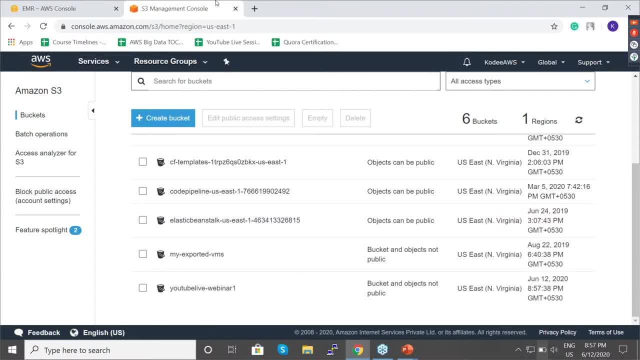 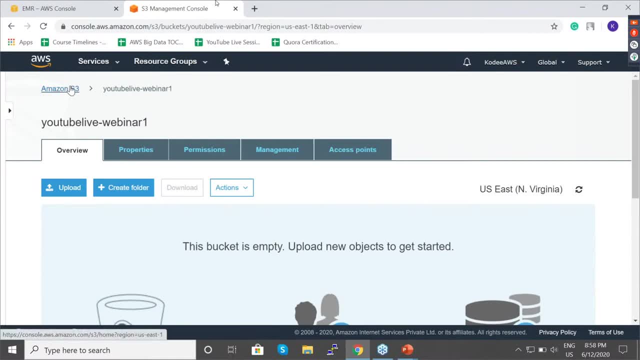 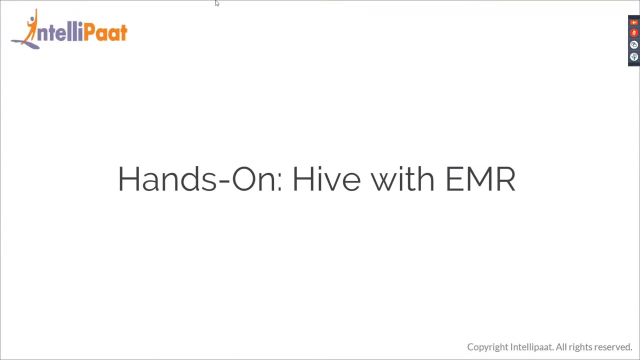 video, audio- all kinds of binary files can be stored here. so we've created a bucket so you can see there's an upload option as well, but we're not going to upload anything over here right now because this bucket is for our output. okay, now let's start with emr. but before starting off with emr, 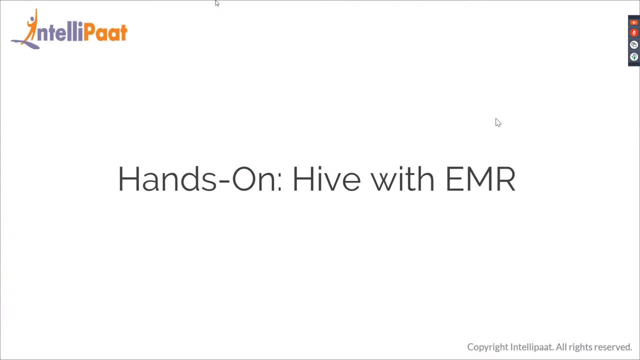 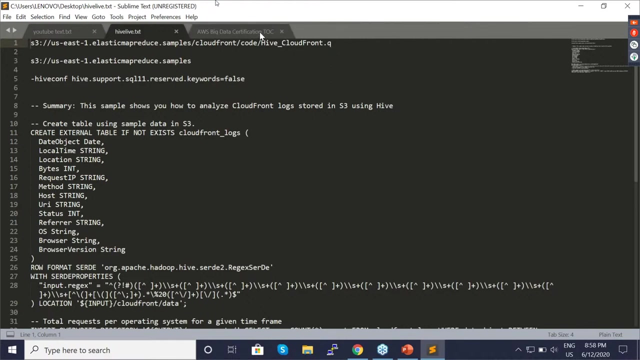 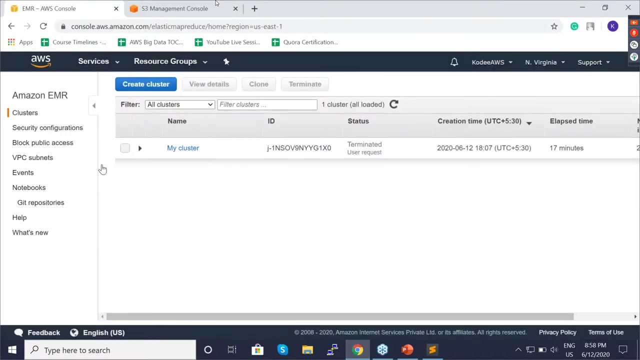 i'll just get a file one second, yeah, so the file is over here. just a second. i'll just close these. yeah, okay, so we are going to create a cluster. so while creating a cluster, i'll be explaining that. so first of all, to start on with emr, get yourself an aws account, but there is no free tier in emr. so 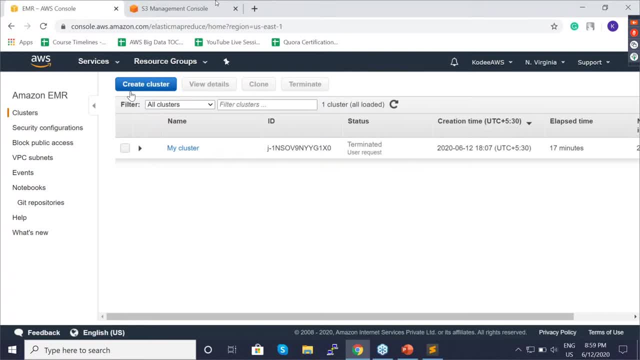 there will be a small charge. it will be around, let's say, 0.04, something like that. it will be a very small amount, so you can go ahead with that, but make sure that you terminate your cluster immediately. so just a second, guys. i'll just get some water. 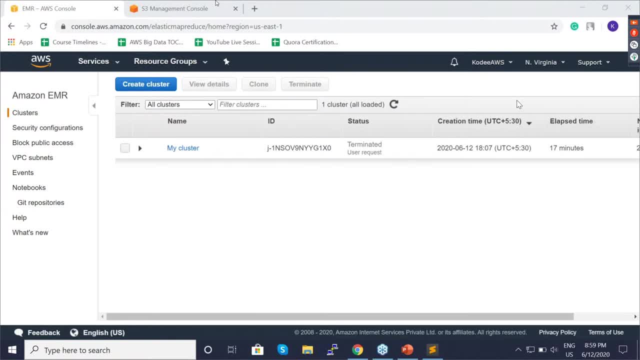 okay, guys, let's- uh, let's- start off with this. so create cluster. so first of all, to start off with emr, as i told, you get an account, then you can start off with this. then come to amazon emr, go to clusters, click on create cluster. okay, so now it's the simple setup. okay, so now it's the simple. 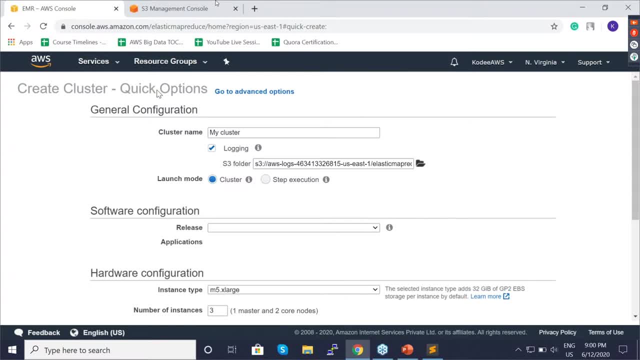 setup. it's very, very simple. yeah, okay. so first of all, you give your cluster a name- i'm going to name it as webinar cluster, okay, and then let logging be on. logging in the sense: whatever happens, the setup, the, let's say, the configuration, everything will be loaded and it will be stored in this folder. 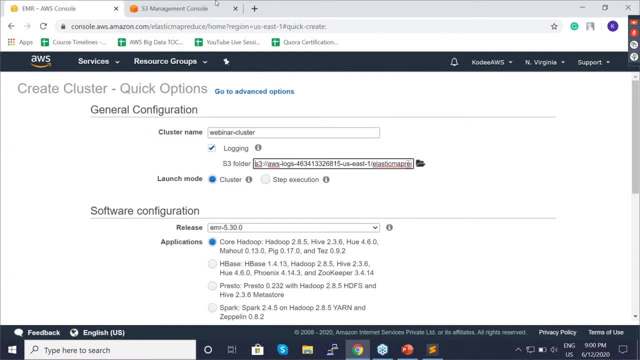 so it will be stored in this folder, in s3. so let it be. why these columns and folders are related to streams is because they are both available in s3, so let it be in s3, in article bar um also. it's very simple setup. it's very, very simple. 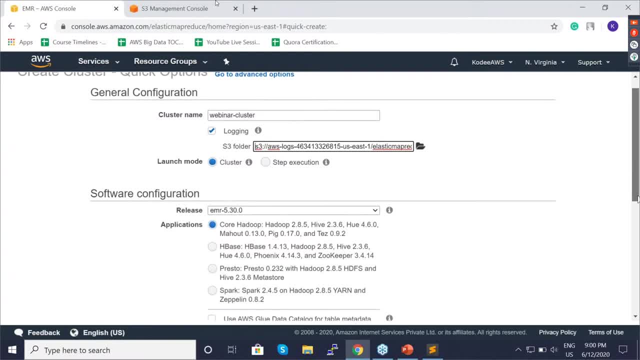 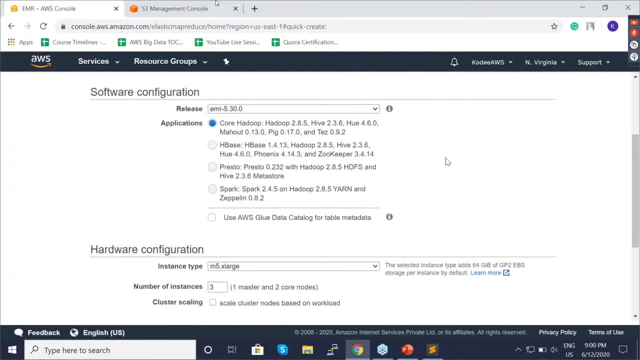 that's fine next coming down. so this is going to be cluster. we are going to start with a cluster and software configuration. so this is where you'll have to choose guys. so here you can see code hadoop. that is hadoop, hive, view, mahout, pig and test. so anyway, we are going to only use hive. 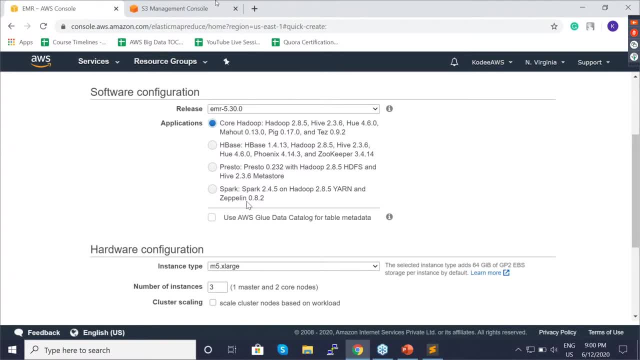 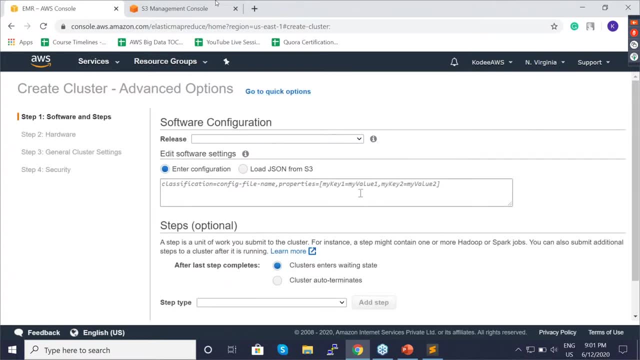 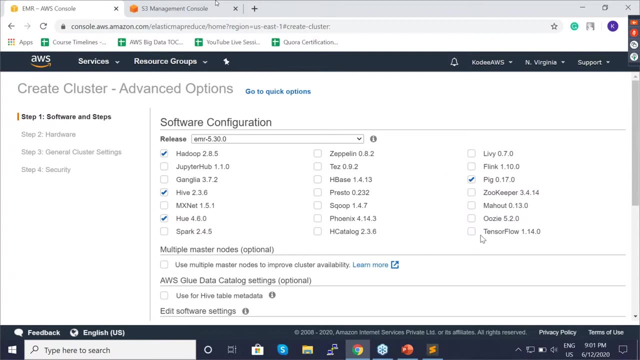 so i'm going to choose first one. then there is for hbase, presto and spark. if you want more options, if you want to choose multiple services, you can click on, go to advanced options and so and you can see here you get to see all the available applications. you can choose whatever application. 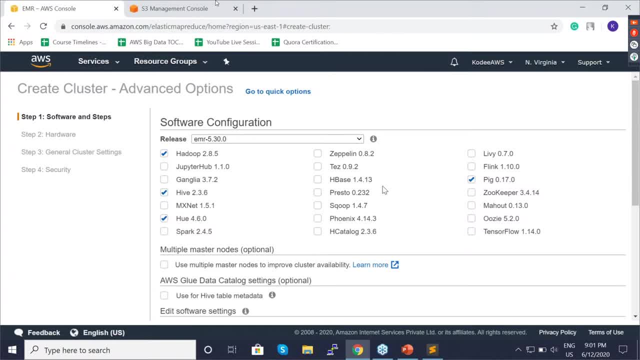 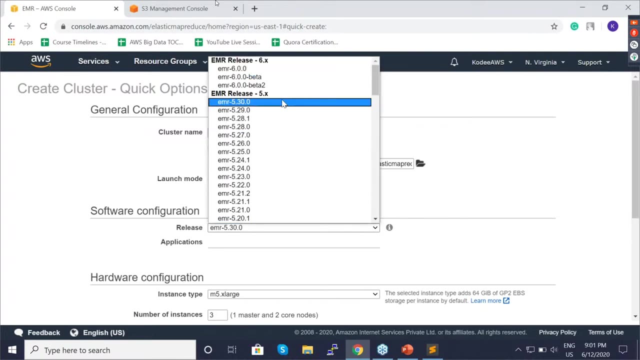 you want, example, tensorflow zookeeper, if there is kafka, then there is flink test. you can choose whichever you want and then you can set it up. but right now we are going to go with quick options because it's easier to understand. at the start, you, so it was the same, so i'm not going to change anything and so you can see, yeah, so i'm going. 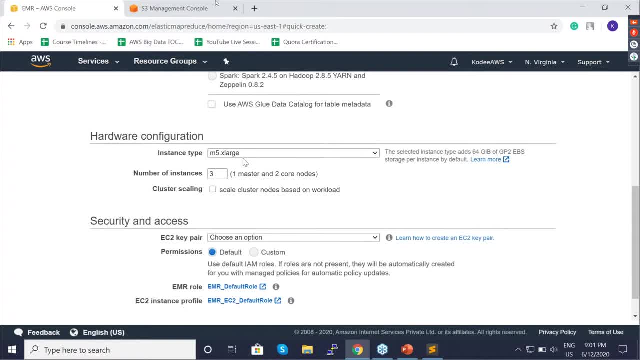 to go with code hadoop and this is the most basic instance type in emr. so let it be, and the number of instances are going to be three. there will be one master and two core nodes, which is basically one master, two slaves. so that will be a master- slave architecture, and then i'm going to choose. 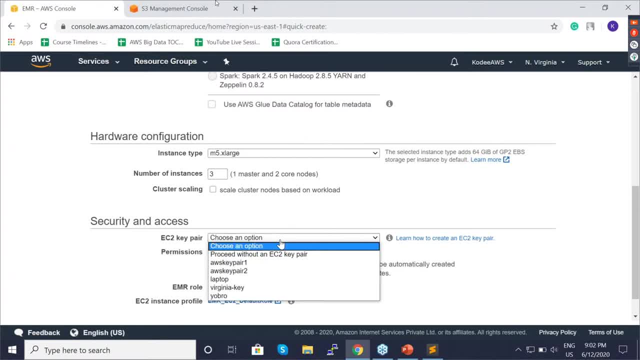 an ec2 key pair. anyway, we're not going to use this. but if you want to use this, you can do that. if you want to log in to the hadoop system and check out what is happening inside of it, you will need this. but anyway, we're not going to open it. but still, i'm showing you. 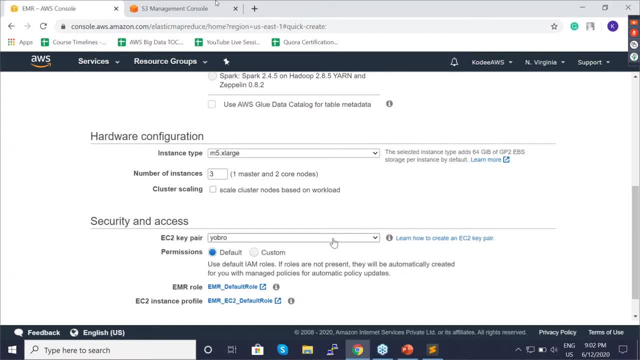 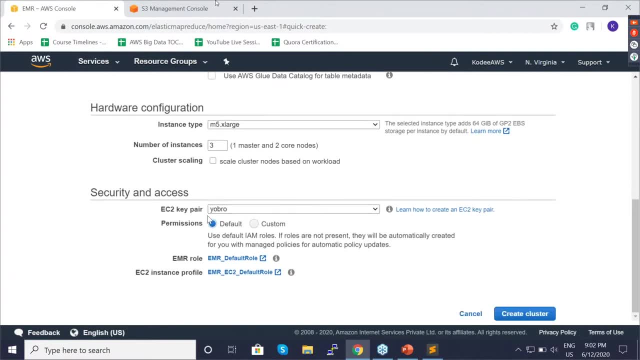 so key pair. you can learn about the key pairs and how to log in with a key pair from our other aws tutorials in our youtube channel. you can check that out, okay. so, uh, this is my keeper and choose a permission. i'm going to go with default. 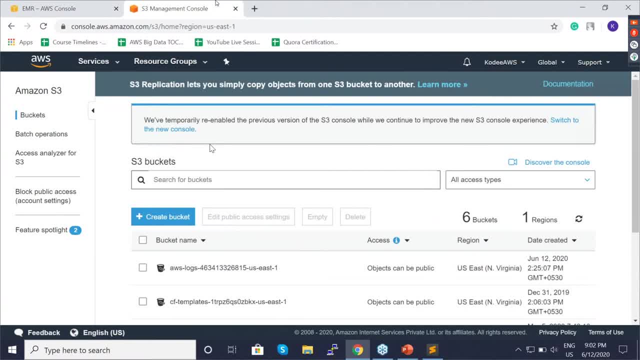 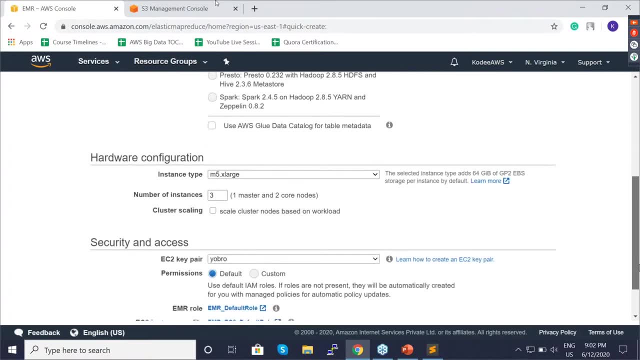 because it's already configured, as we will be taking the data of uh, pushing the data into s3, so i'm going to go with this. uh, yeah, okay. so now you can see this and if i hit create cluster, it will start, but i'm not going to do. 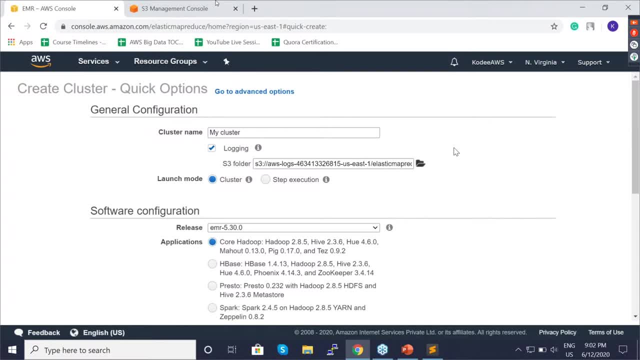 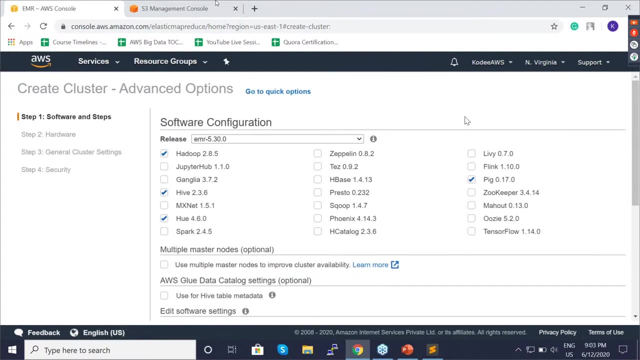 because i'm going to go and do this exact same thing in advanced options. i think i understood this part. if i click create cluster, it will create a cluster. so there's there's one small step in this, that is, we'll have to uh mention the input data and the output folder where the uh result. 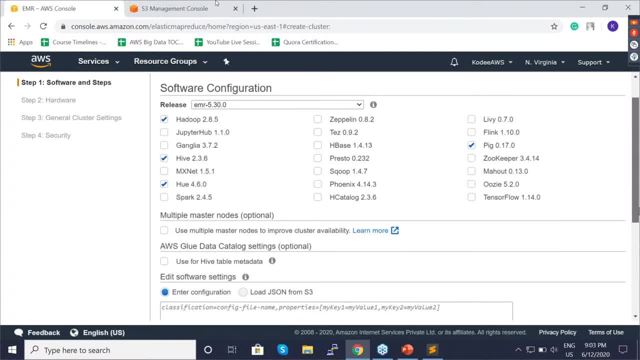 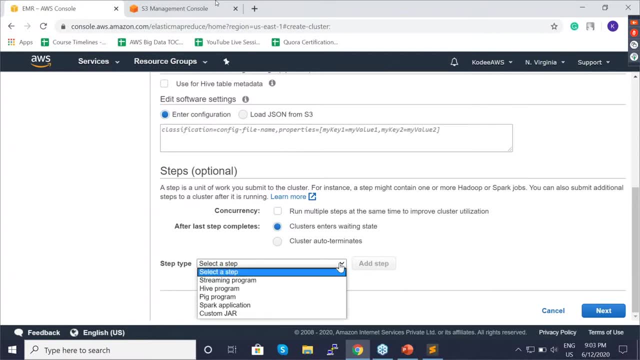 has to be stored, so i'm not going to make any changes. it is going to be the exact same configuration. i'm not going to change anything. the only change we'll be making is adding a step. so our step would be a hive program, because that's what we're going to do. we are going to include a 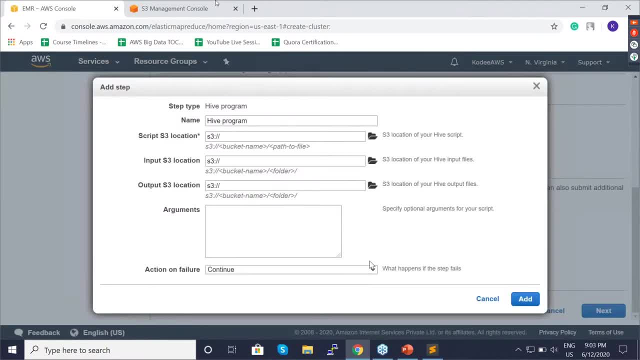 hive script. so i'm going to click that and i'm going to click add step. okay, so you can see script s3 location. so we'll have to provide the location of where the script is available, then we'll have to provide the s3 location of the input files and then we'll 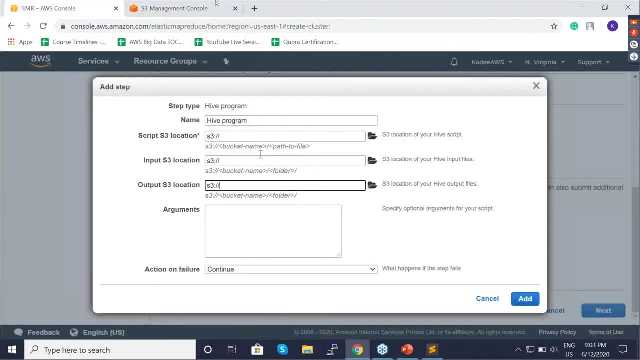 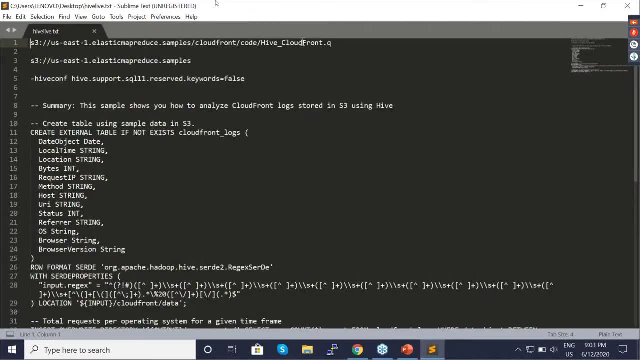 have to provide the output location which we created, okay, and an argument, okay, so that is fine coming down. so this is what i wanted to show you guys. so if you want to check out this, you can just go ahead with the documentation provided by aws for amazon emr. so this is one of the tutorials they provide. so this is the crypt link, so the script. 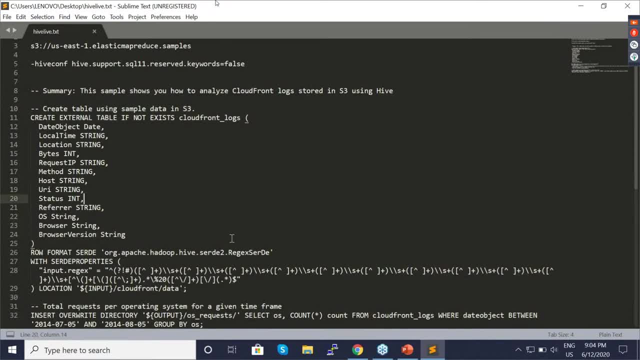 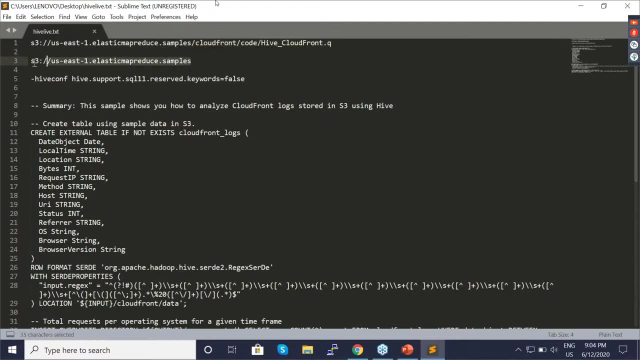 is over here. i'll explain to you about this. this is the script, this is the script link and this is the input folder. so, as you can see, this is the input folder of the s3 bucket and inside this bucket there is a sub file called cloudfront. inside that there is a sub file called code and inside that there is the. 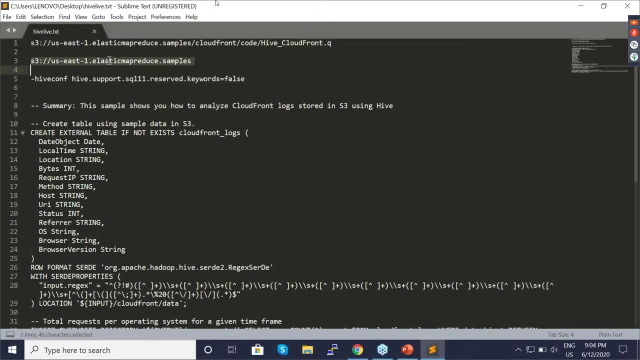 crypt file. okay, that is fine. and then there is the input. okay, and this is basically a command which aws told to add in the argument section so that if there is any uh keyword mismatch, it'll automatically take care of it. okay, that is fine. next, coming to summary. so this is the script which 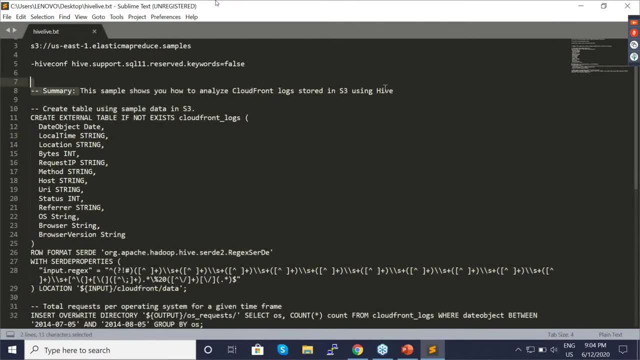 will be running in hive. okay, so you can see this and this is pretty much. pretty much it's going to wrap it up pretty much in the end. pretty much you can see that we are actually потерquer pretty much it what exactly we are doing right now. so this sample shows you how to analyze cloudfront. 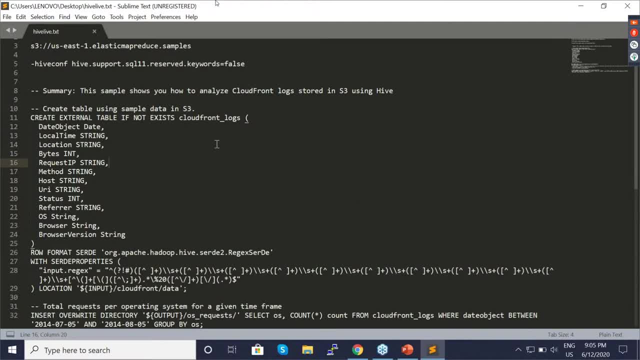 logs stored in s3 using hive. so we are using hive on emr to analyze logs which are generated from will run. this script will process the data and give us the output and we can download it and check the acquired results. so to check that, first of all you'll have to set it up and before that 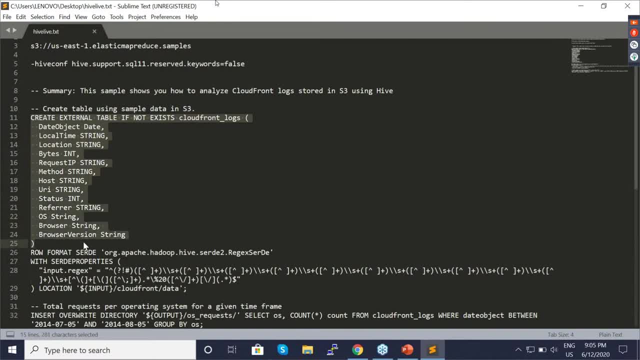 you can see over here you'll have. so this script is creating a table, so it's creating a date. it's you can see local time, location, bytes, host, os and browser. so what we're going to do is we are just going to get the count of the os inputs. so, coming down you can see total requests per operating. 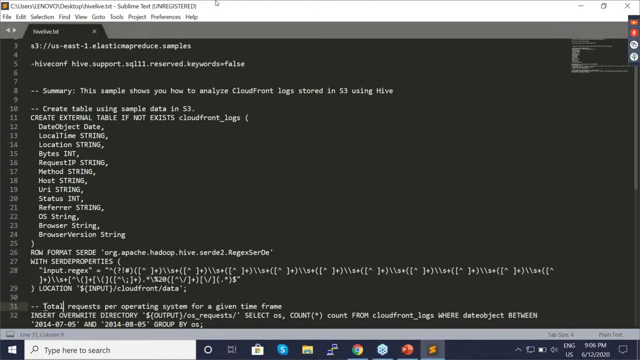 system for a given time frame. so what result we are going to get is, for example, there is mac os, there is windows, there is ubuntu, then there is android, so all of that operating systems. so let's say, in cloud front there is an application running, so cloud front is basically cdn. okay, 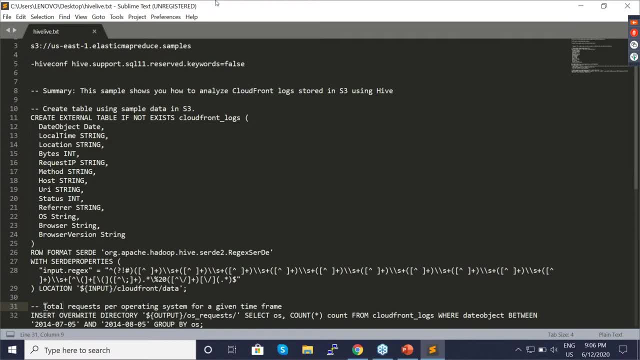 so there is. so let's forget about that, let's just concentrate on this. there is an application running guys, so that application could be accessed from all kinds of operating systems: from a windows system, from a mac mac system, that is, an apple laptop, or from an iphone, from from a safari browser, which is an ios. then 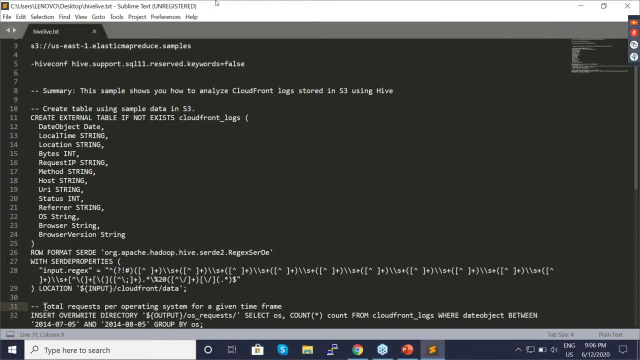 there is ubuntu, then there is android, so that application could be accessed from all these operating systems. so the output we'll be getting is how many hits were from each windows or mac or any operating system. so the output would be the operating system and the number of hits. this 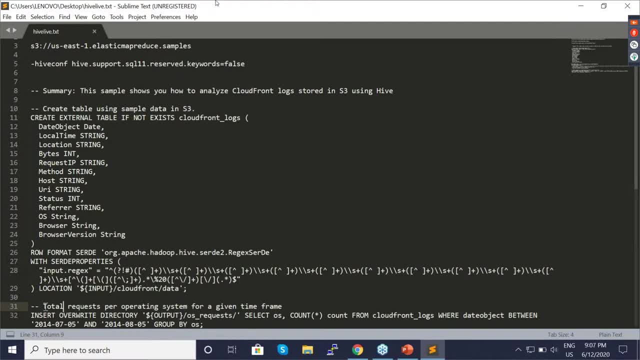 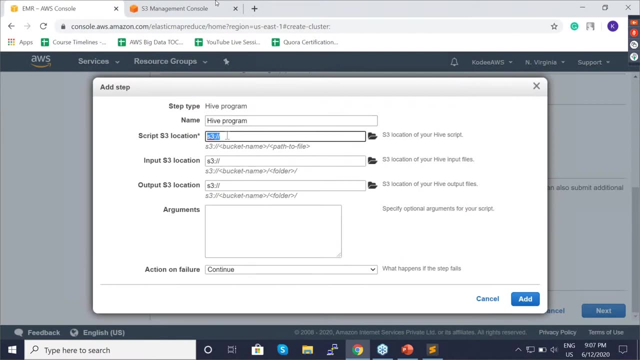 particular application got from that operating system, so this data is already available, so it's not going to be dynamically changing. it is static data. okay, so i think i've explained to you this part. now let us start off with configuring this. so first of all, i'll have to provide the s3 location. 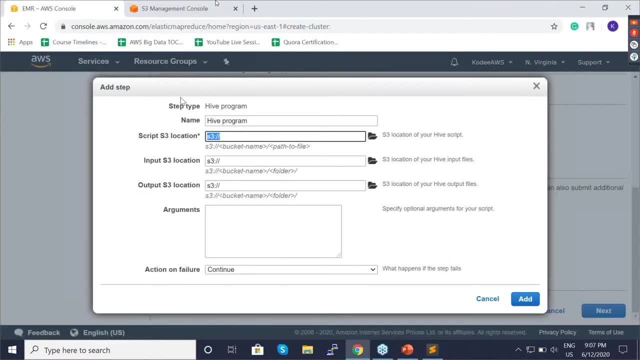 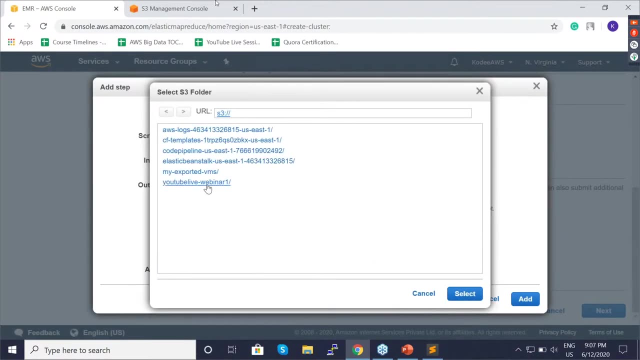 so this is the s3 location, so i'm going to provide this done. next is the s3 input location, which is this. i'm going to provide this. next would be our output s3 location. so for this we can search over here, and this is the bucket which should contain our output files. 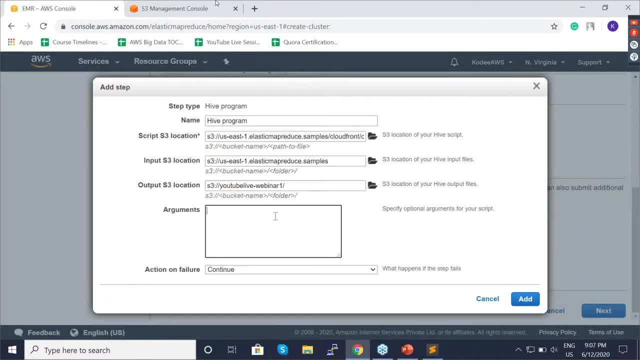 so i'm going to click it, select- okay. next is the argument. i'm going to copy this and paste it over here. just a second, guys, i'll just get some water. Yeah, So now this action on failure is: if this particular code or this particular process fails, it should continue and create this particular cluster, or you. 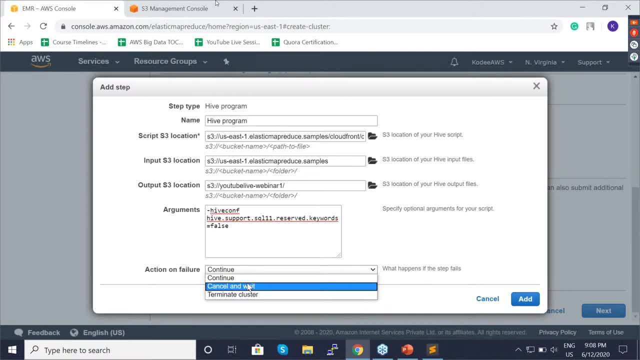 can cancel and wait. So basically the cluster will be stopped and then terminate cluster. If this particular little for this script we are running fails, then this cluster will be automatically terminated. if you give terminate cluster- but I'm not going to give that, I'm. 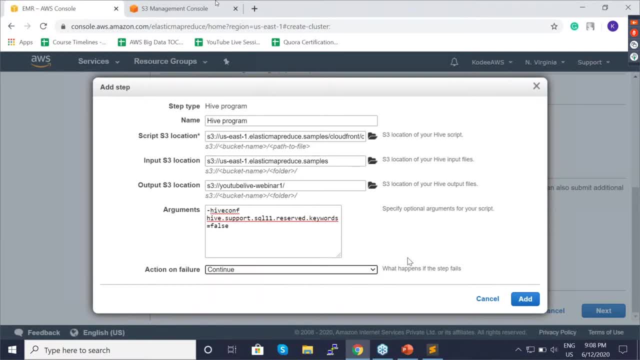 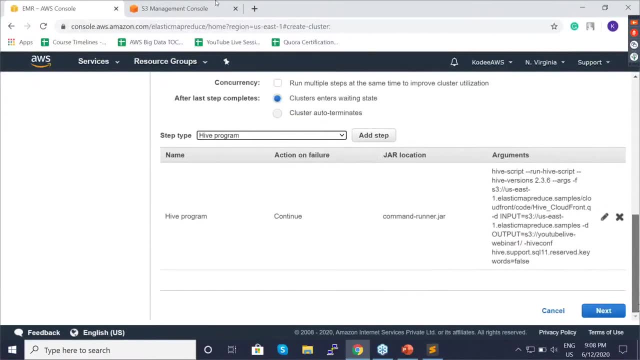 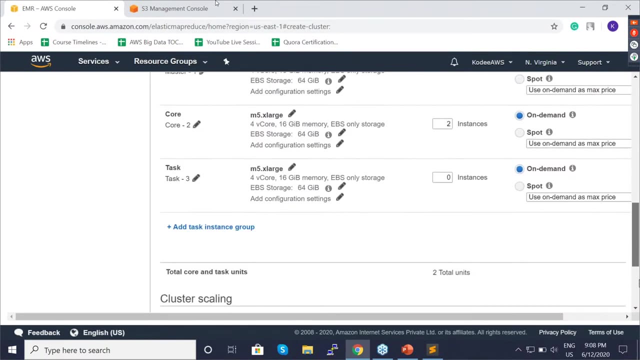 going to give continue. If this step fails, our cluster will still be active, So that's what it means. So now I'm clicking on add And you can see we have set this up. That is the only extra step I'm just going to give next. Next, I'm not going to change. 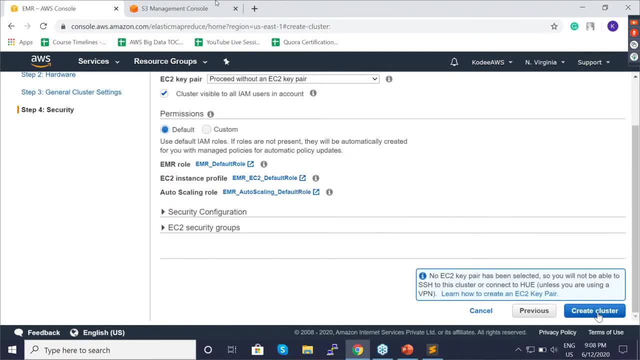 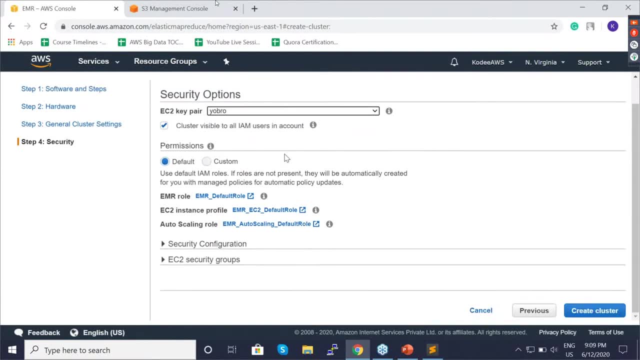 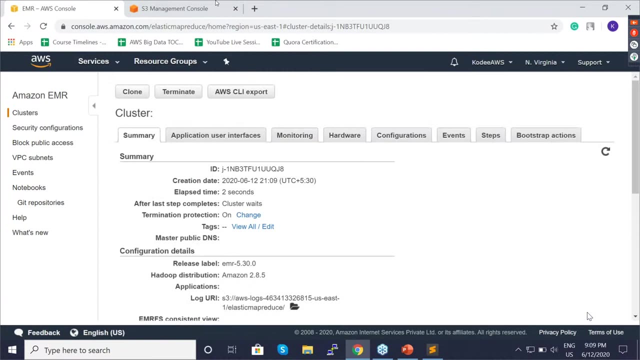 anything? Yeah, so you can review it once So you can see it is proceed. without an easy to keep it, I'm going to give my keeper and create cluster. So, guys, it will take from five to 10 minutes to create this. So you can see the steps over here. 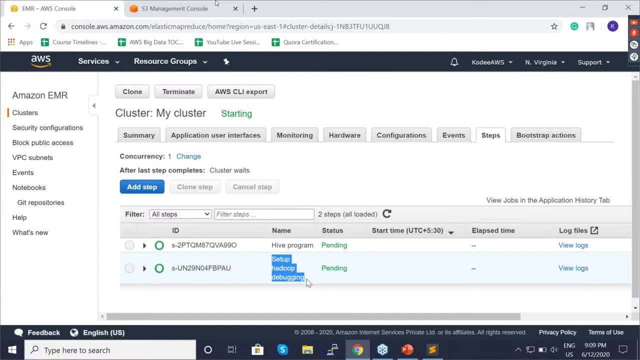 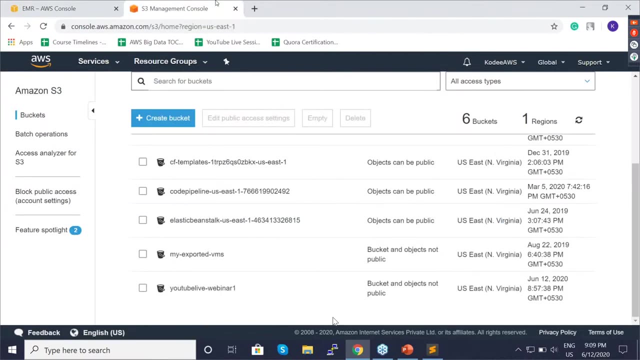 You can see, first, this step will be completed, That is, the setup will be completed. then Hadoop and debugging, everything will be completed. Once that is done, the hive program will start running within the cluster. Once that is done, we'll be able to see our output in this particular 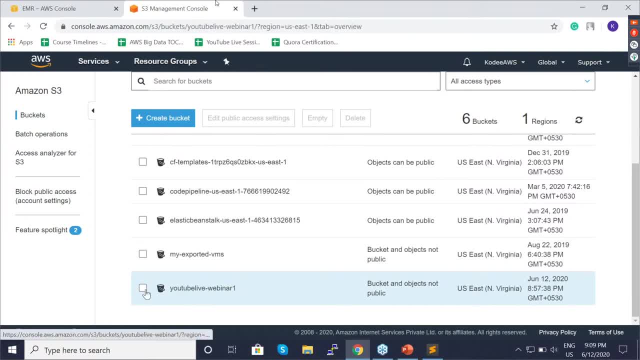 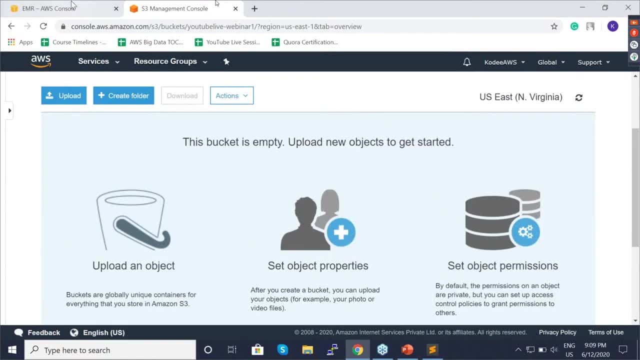 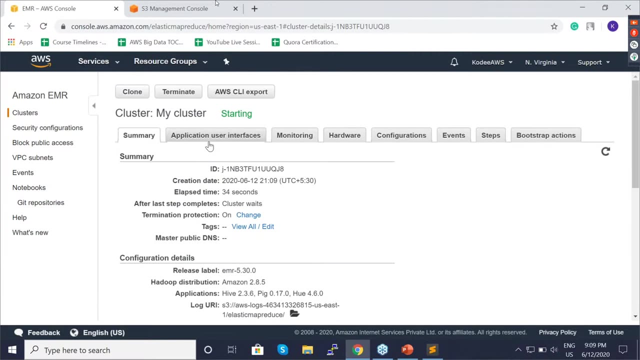 bucket. So if I open this bucket right now, you'll not be able to see. Let me just refresh. Yeah, so I'm inside the bucket. So right now there are no files inside this bucket. Once this is done, We'll be able to see that. So, as I told you, it'll take some time. So let me go to let. 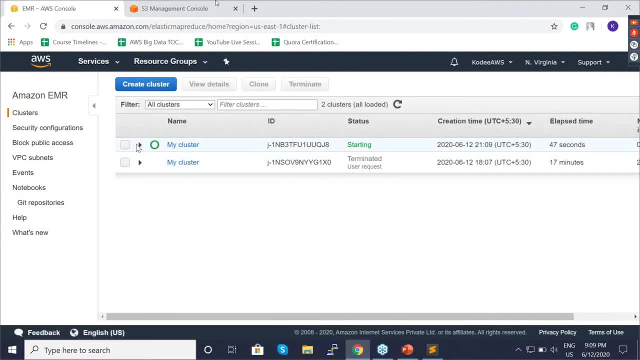 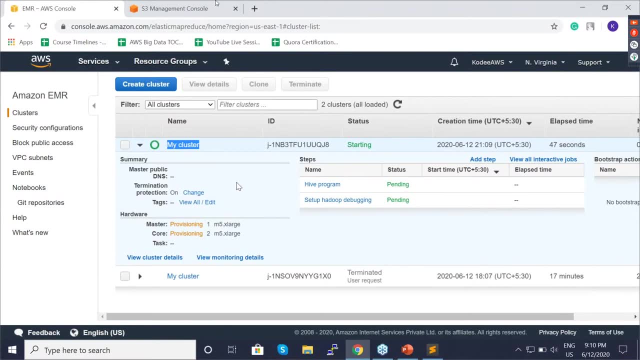 me click on clusters Here you can see I already had a cluster which I terminated. So you can see it is my cluster, because once I went into advanced options I did not change the clusters name So it was my cluster only. So it's the same. it is right now starting And once we 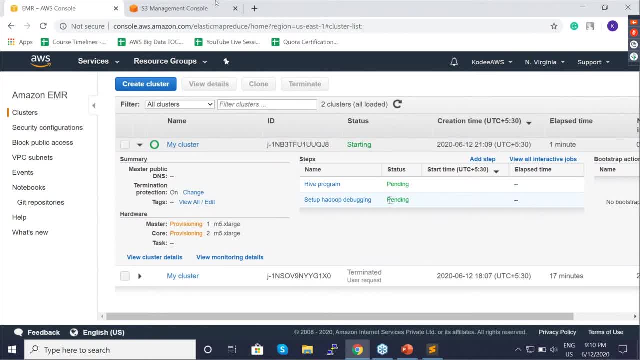 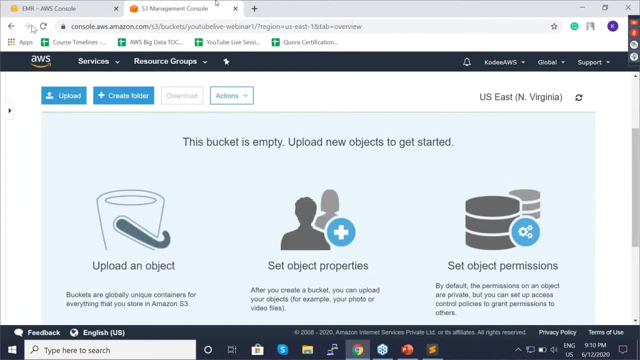 see complete over here, then this process will start, And once this is complete, we'll win, Because once we see complete, we can see the output, And after that this process will start, And only then we'll be able to see the output. So then we'll download the. 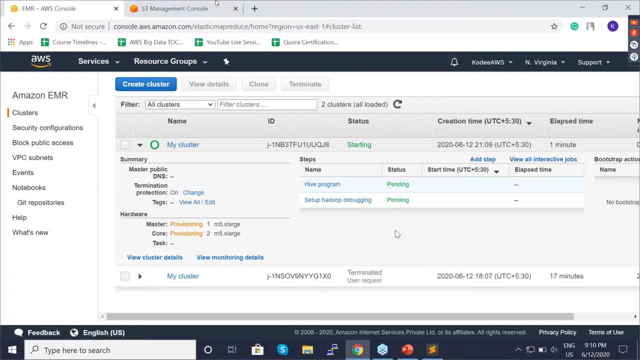 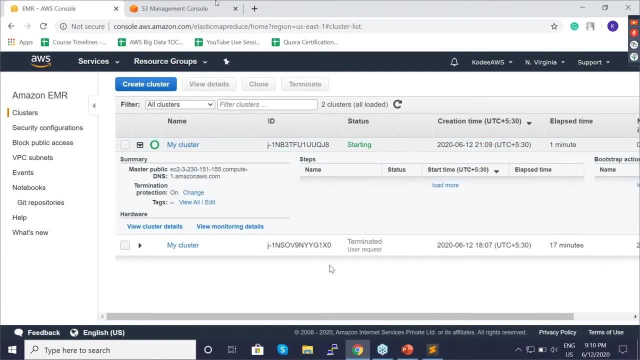 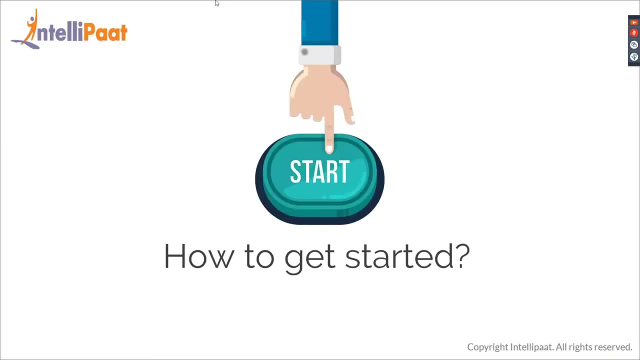 file and see the output, guys. So I think that's clear right now. So the thing is will not be. we're not going to wait here and just sit idly. So I'll just finish off the last part of the session and then come back to the hands on. Let me go back to the slides. So 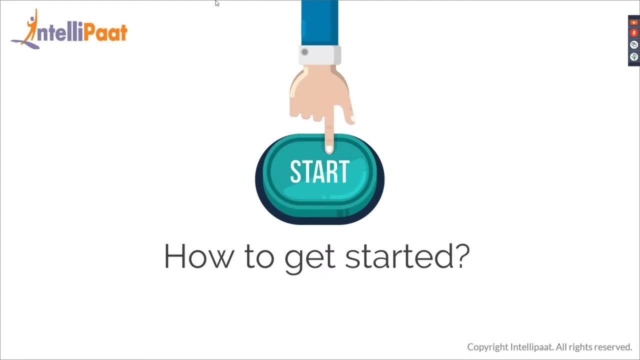 how to get started with anything or any technology. In our case, it is AWS on big data. sorry, big data on AWS. Okay, go ahead. Okay, let me go back to this. Let me go back to this. Let me go back to this. 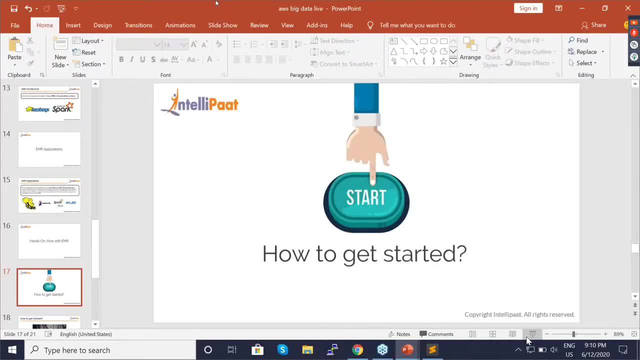 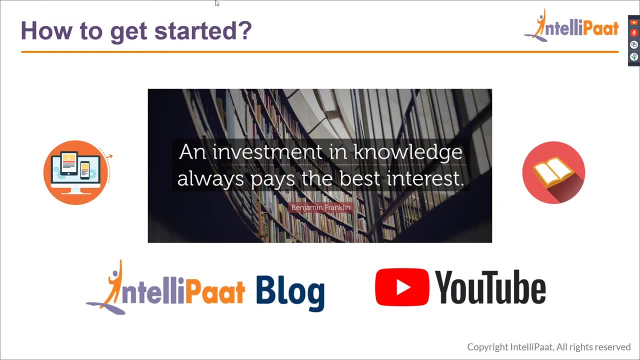 AWS. So the thing is, we at Intellipaat, we provide you a lot of free resources. You can check out our blogs. You can check out our YouTube channel, which has a lot of free content. There's a lot of courses. You can check out our AWS course as well and get started with your AWS. 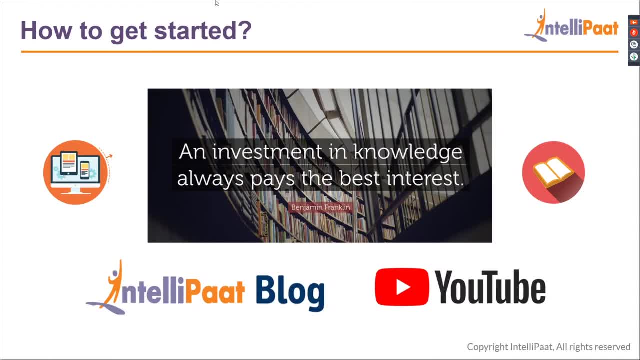 career, So this is one which you can start. The investment is not always money. It can also be your time. So put in your time and you can get some knowledge out of it. And then comes our Intellipaat Academy, which we have recently introduced, And this is an online academy. 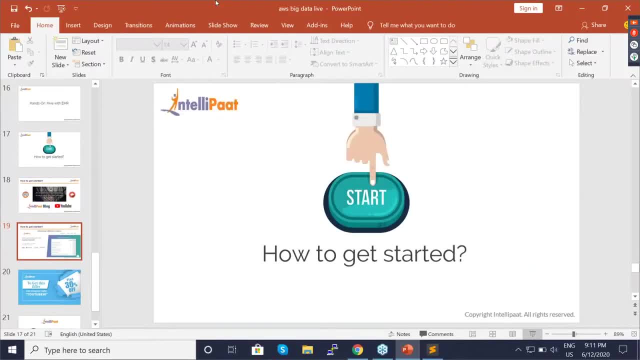 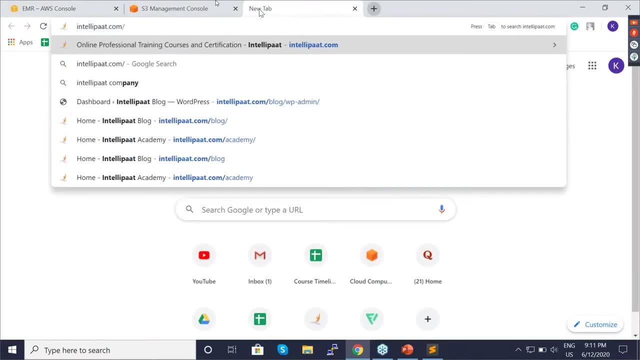 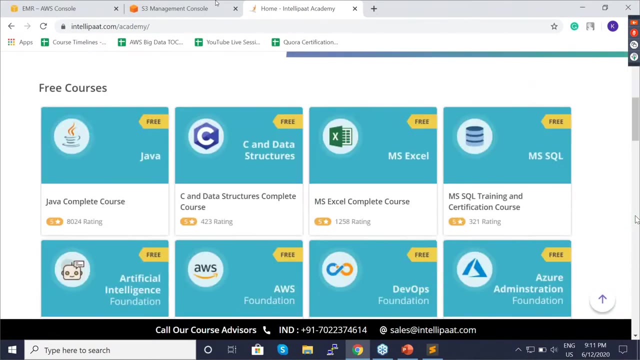 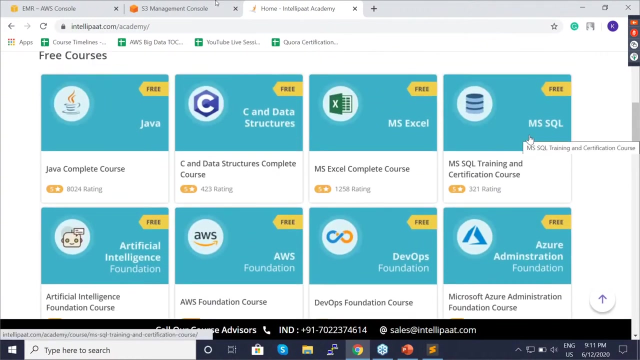 which provides you free courses. So let me show you that. So just go type in our initial website: slash academy. Yeah, So once you're in, you can check out, You can come down, you can check. we provide a lot of free courses. you can see there is java c, ms excel, ms sql. then 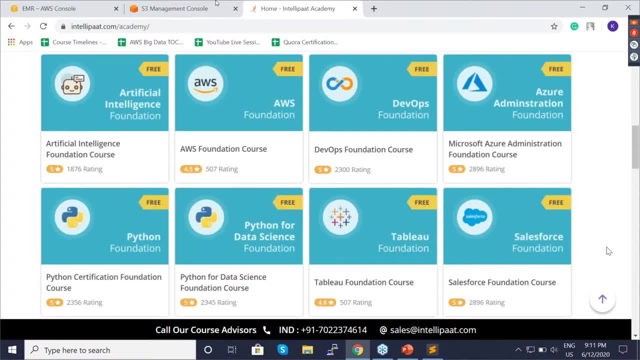 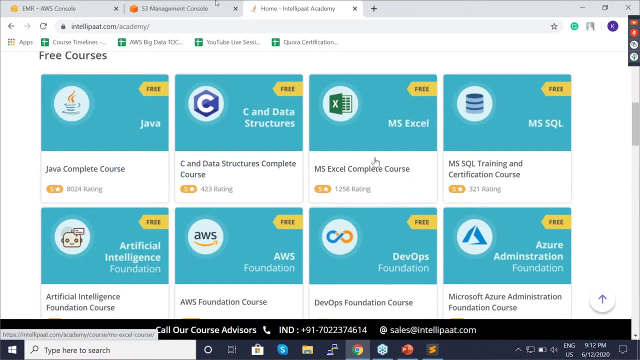 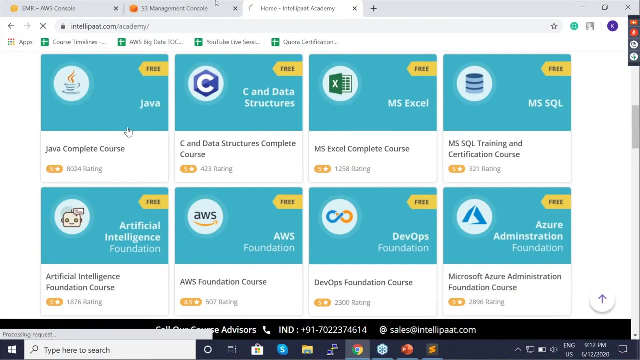 there is ai foundation. so mostly these courses are foundational courses which you can start up and learn a lot about, and then you can also take the java full course, the c full course, ms excel and also ms sql training. so it's pretty simple. let's say you want to start off with java, come over here, click on the course. click on, take this course. 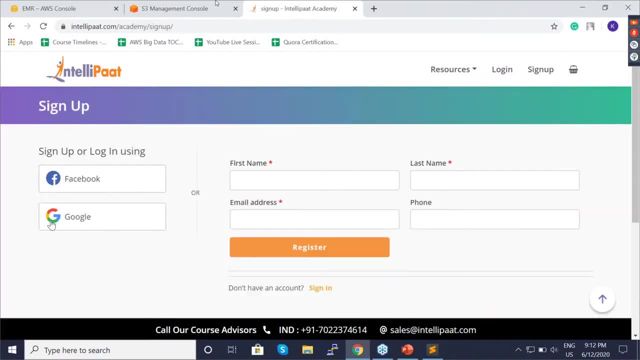 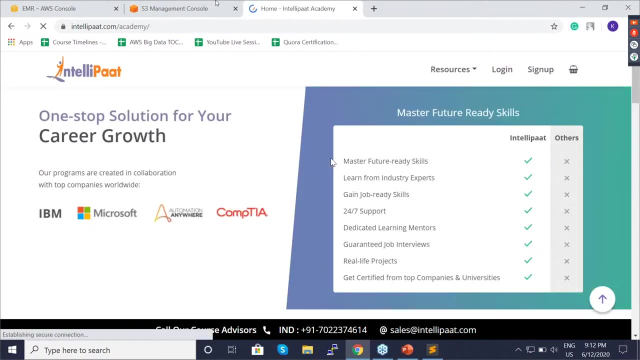 and you can log in using a third-party login- uh, google or facebook- or you can just provide your first name, last name and email and then click on register and that's it. it'll be done, okay. so this is one of our resources if you want to check out aws courses. so, right now. 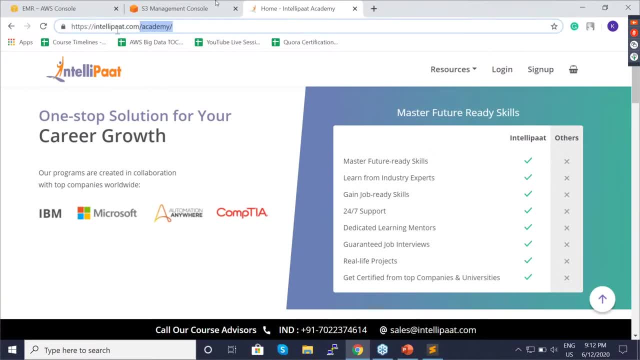 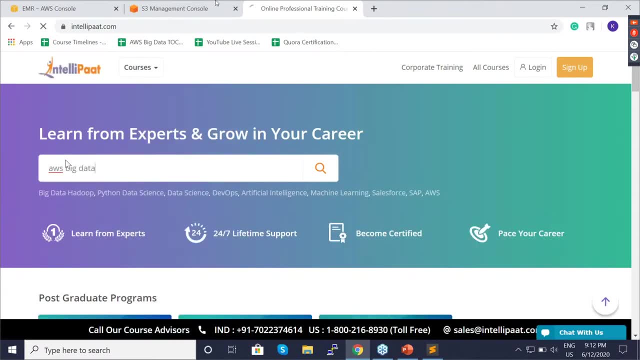 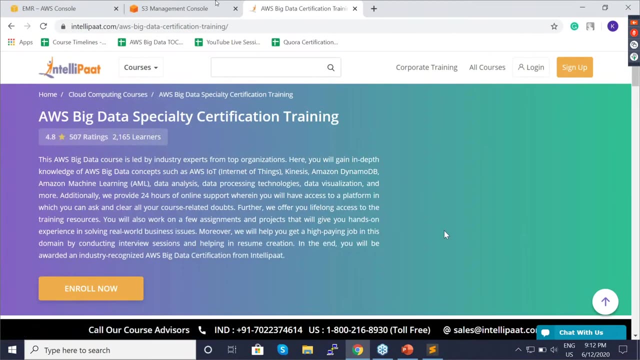 we are coming up with an aws big data course as well. if you want to take up that course and get training from industry professionals, come to our website. just search for aws big data and you can get that training page and you can get over here and you can enroll already. you can check out the course content. 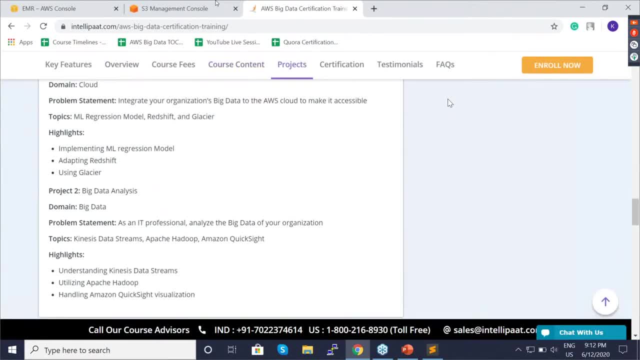 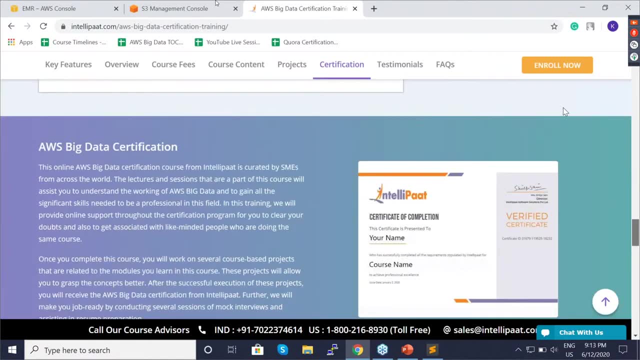 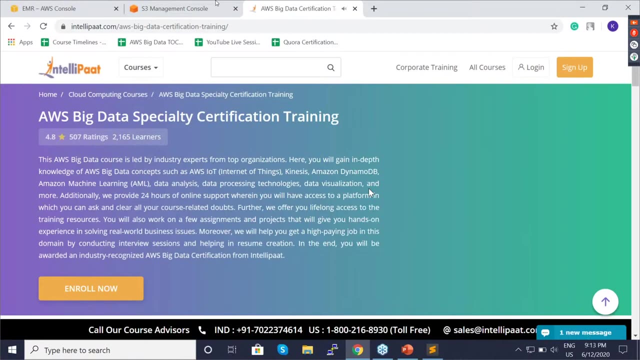 from here, you can see all the course content coming down, you can check the project which we'll be doing and you can check out the certificates which we'll be providing. okay, so this is our aws- big data speciality certification training. you can enroll with us and start off your big data career using aws from here itself and also, if you want to contact us, you. 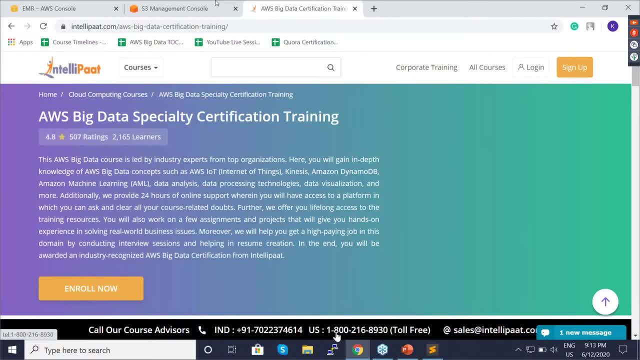 can call us from this number if you're from india. if you're from any other country, you can call us in this toll-free number, or you can put up a mail to sales at intellipadcom and we'll get back to you immediately, or you can just come to our website and start conversing with our 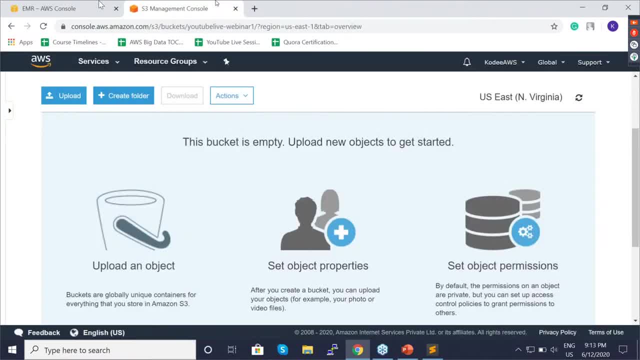 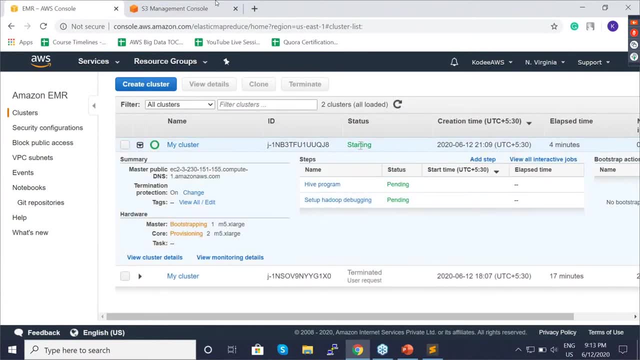 chat agent. okay, so that's done, let's go back check whether it's still pending. yeah, it's still working ahead, so this process is still starting. as i told you, it will take from five to ten minutes to this getting completed. the thing is, we added a step before we launched. you can also add a step. 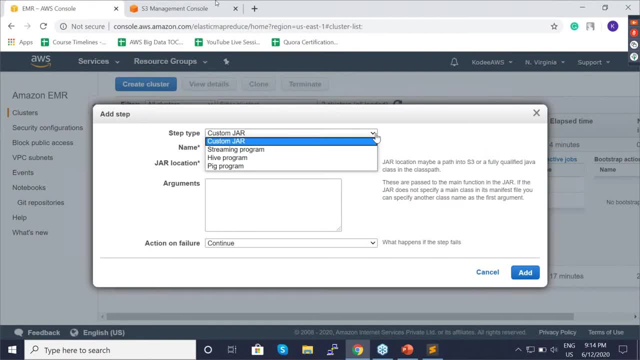 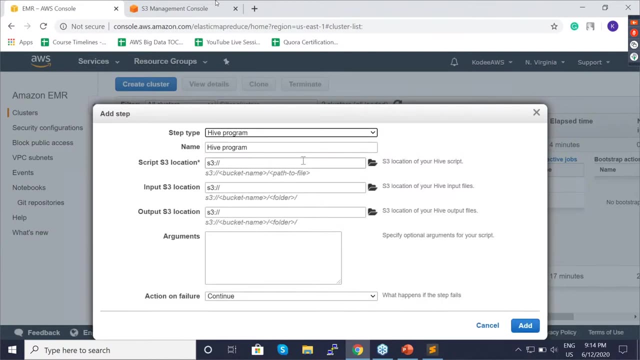 once it is set up, so you can see, here you can also add this. uh, sorry, you can also add a step. once you've uh created your cluster, you can choose a pick program, a hive, a streaming program or a custom jar program. so if you want to add another high program, it's again the same setup. 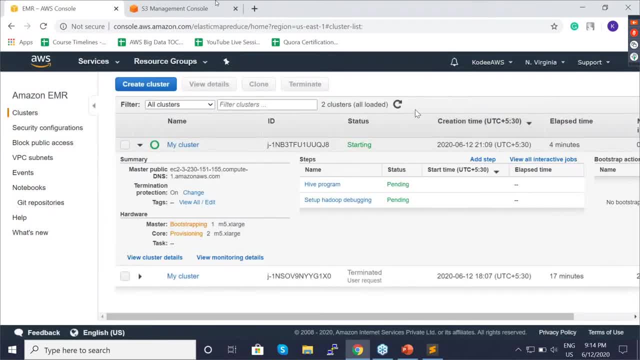 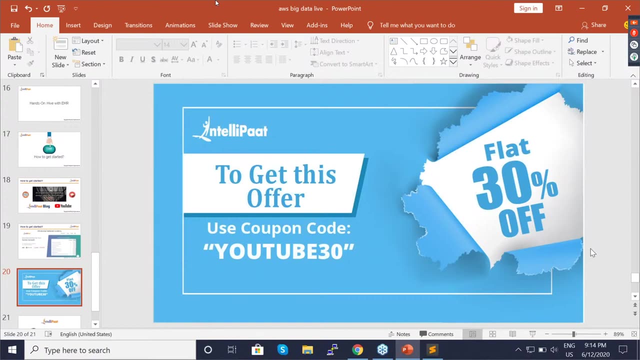 and you can do that. okay, so you've seen this. it's still starting, so there is nothing else to do over here. going back, one more thing, guys. if you're watching this live right now, if you're in this- em- uh, sorry- in this webinar, if you want to take up any course from us, 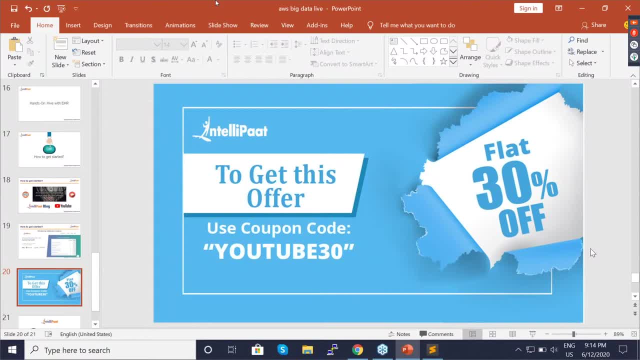 use the code youtube30 and you'll get an instant Represent Capitolis level on your website�� exam given by Digital Building Pandemie再 controllers. you'll get an instant 30% discount and you can take up any course you want. so this is what we want to provide. 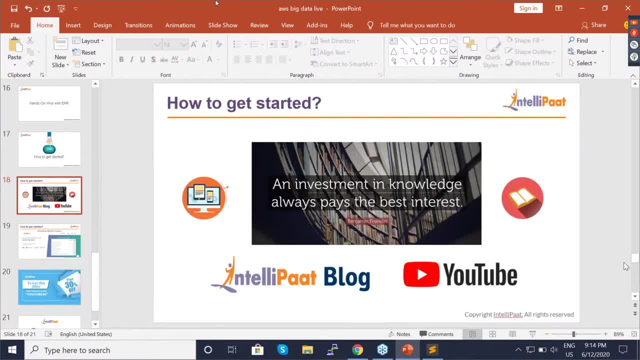 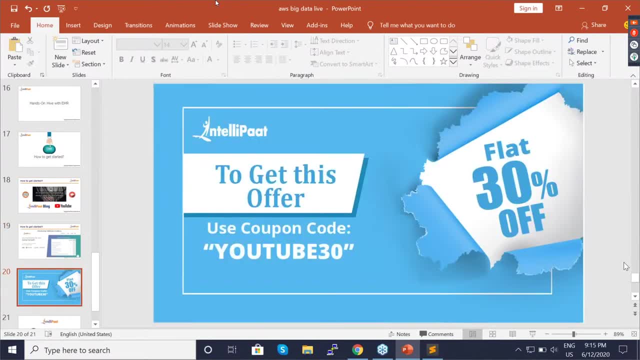 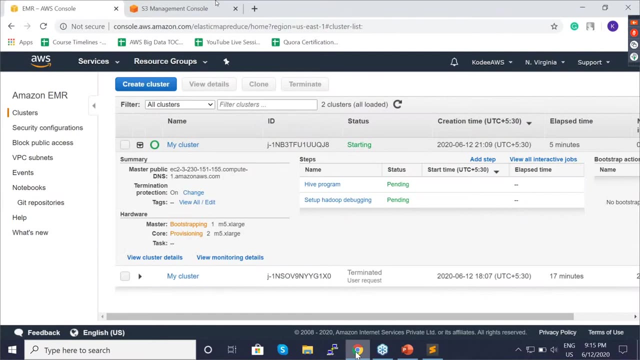 to you. so one would be our blogs and YouTube channel, and we have a academy which provides you free courses. then you can use this on our main website to get 30% discount on any course you want to take up. so okay, we've seen that. the only thing we'll have to see is our 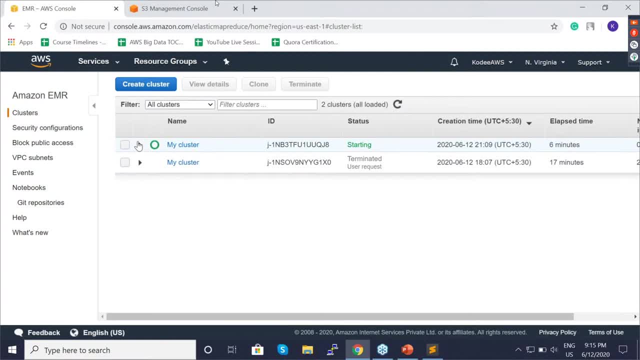 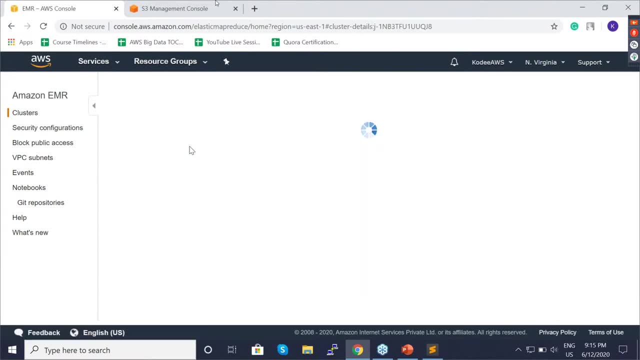 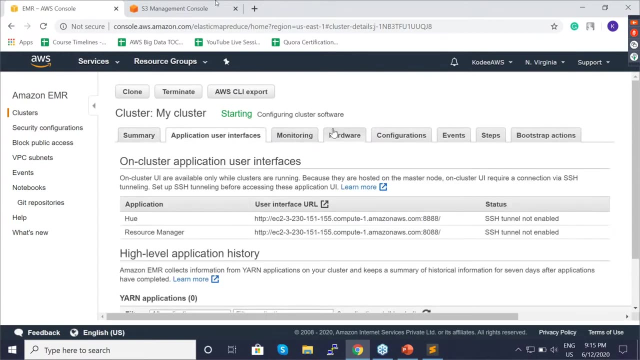 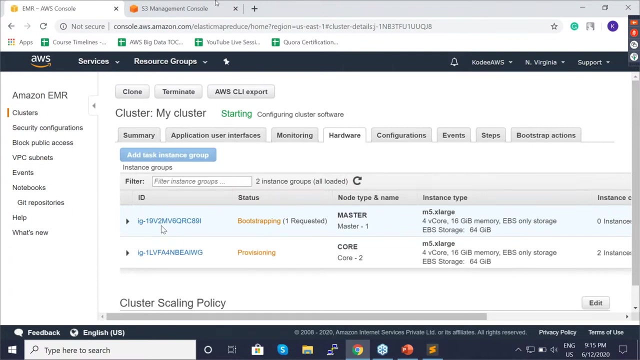 demo completing, okay. so while doing this, I'll also explain the other things about this cluster, because there is no need to waste your time as well, because it's everybody's precious time over here, okay, so, coming to hardware, you can see this because we wanted to launch three instances: one is sorry, one is a master instance, two core instances- you 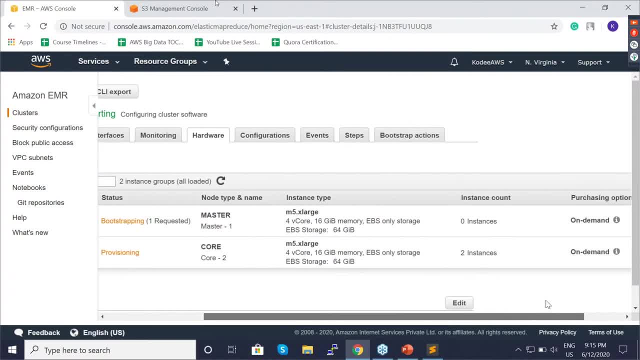 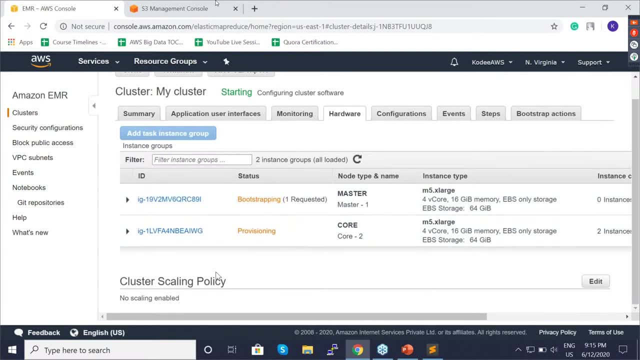 can see the two core instances. you can see the two two core instances are created. the master instance is currently under creation and so right now we have not enabled any scaling policy. let me explain to you about the scaling policy. so it is basically for auto scaling. click on edit, come down so you can see: enable cluster. 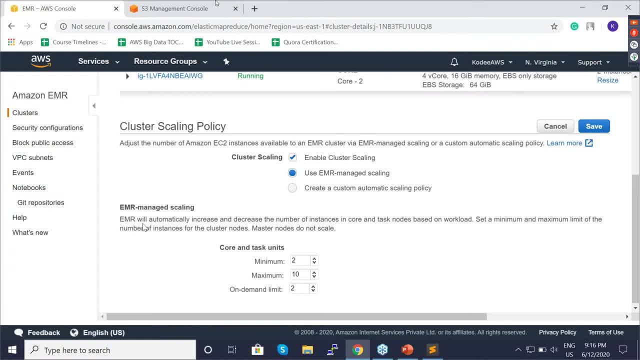 scaling. use the emr, named scaling, so come come over here. emr will automatically increase and decrease the number of instances in core and task nodes based on workload. so if the workload increases, it will automatically increase the number of instances. the workload decreases, it will automatically decrease the number of instances. okay, let me close this. i'm seeing. 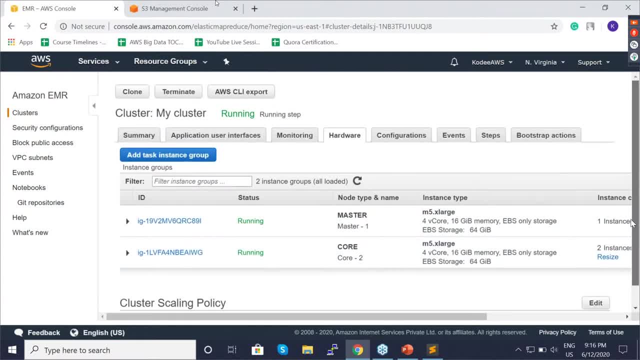 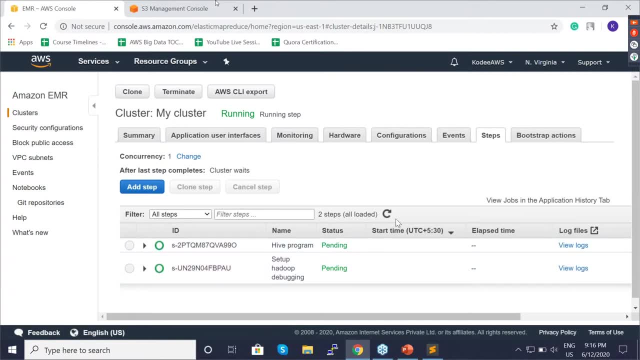 running over here. yeah, so the instances are running, guys, so you can check out the steps over here as well. you can see the instances are running, but the steps are still pending. so now you this step has completed. so once the instance is run, it got set up in four seconds, if you want to. 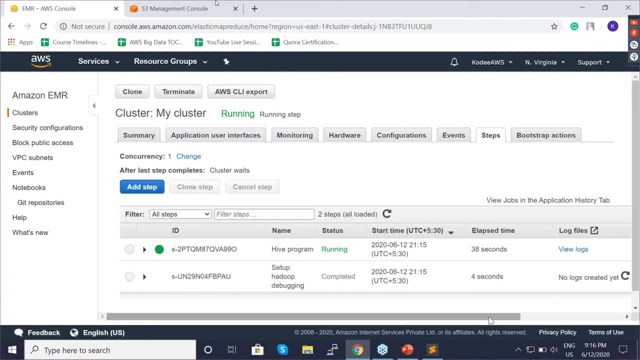 check out this logs, just click over here. so right now there are no logs. so once the log is created you can just refresh and see over here and that logs will be available in s3 and you can go check out those logs. but this step is still running and now it is completed, guys, so let's go over here. 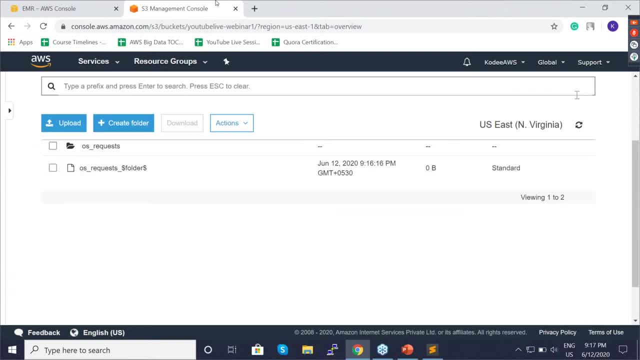 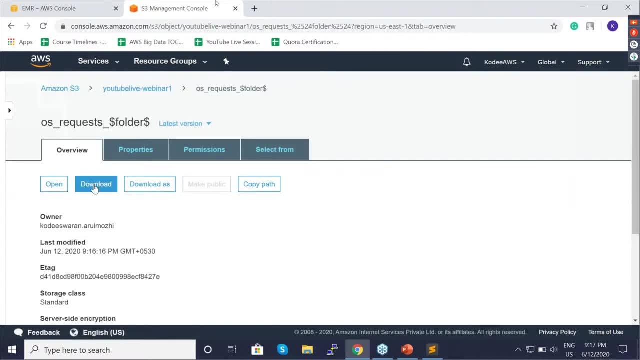 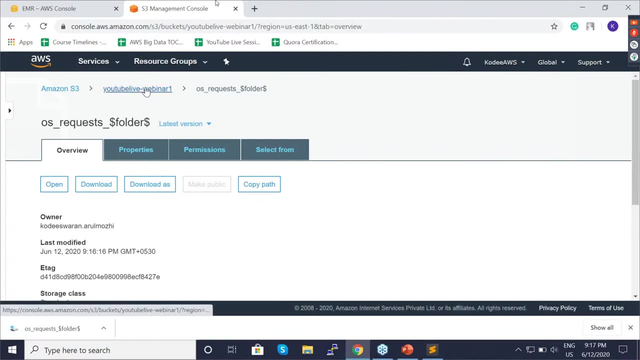 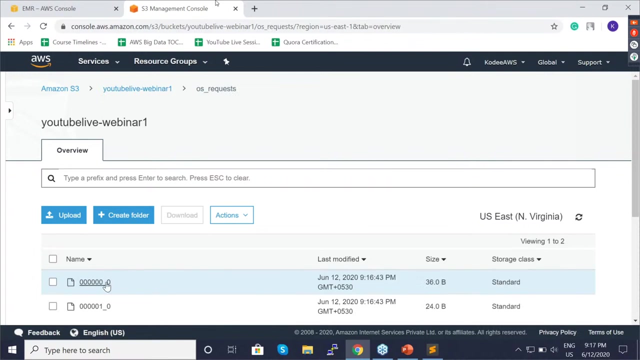 refresh this and hope that we get an output. and we got an output, so let me open this folder and let me download this. okay, sorry, that's not the full. that's not the folder which we want to download. we can download that, or we can go inside and download this. so the thing is we have two nodes. 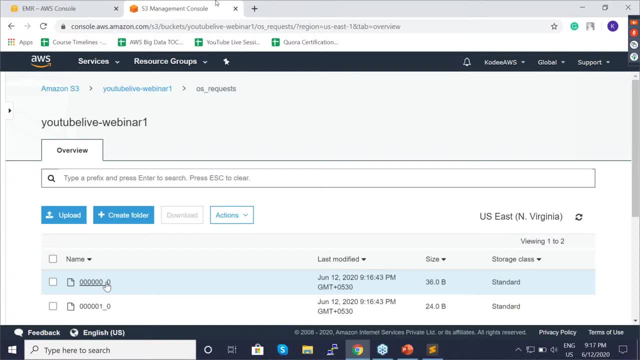 that. so why do we have two nodes? is that we'll be splitting work and giving it to each instance. that is, the half or some of the work will be given to the first instance and some of the work will be given to the second instance. so you see two files over here. so this file would have been 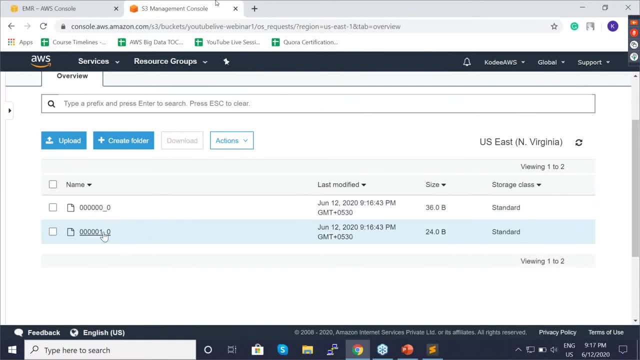 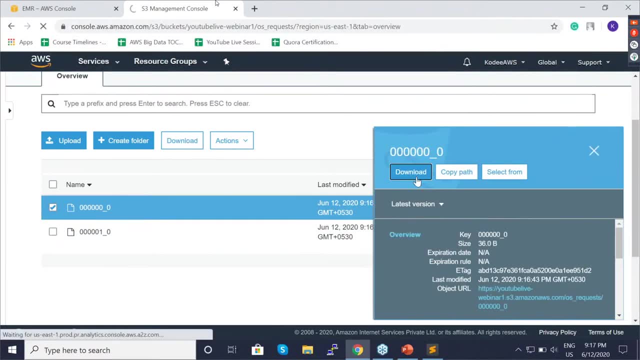 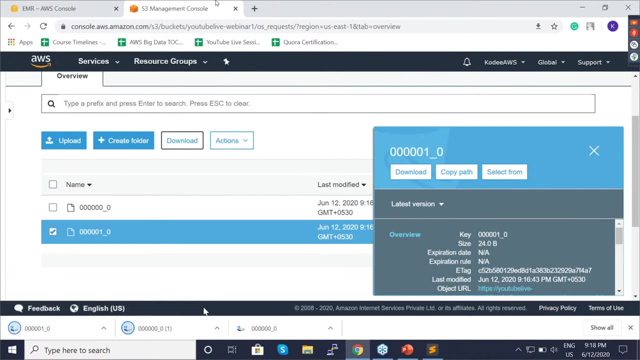 a processed in the first instance, this file would have been processed in this second instance. so now let's download. sorry, i think it's not possible. let me click: download the first one, click and download. sorry, i downloaded it multiple times. okay, so we've downloaded it. i'll go to the folder. 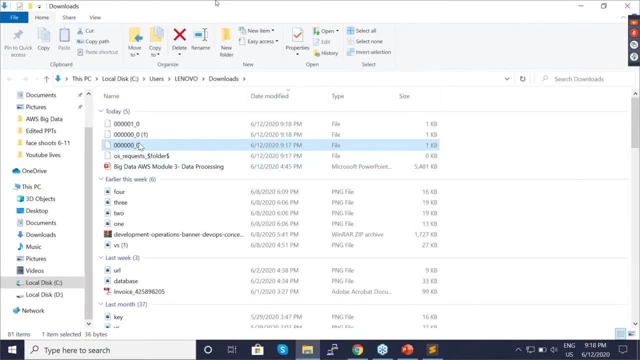 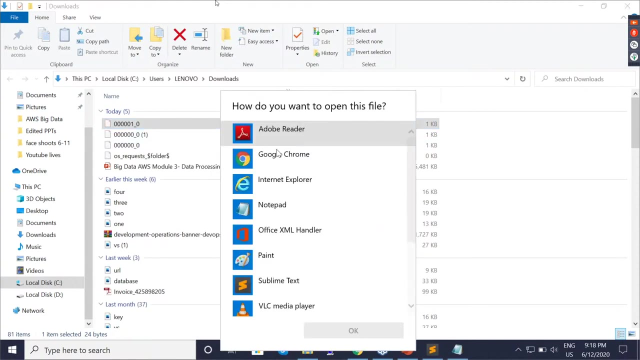 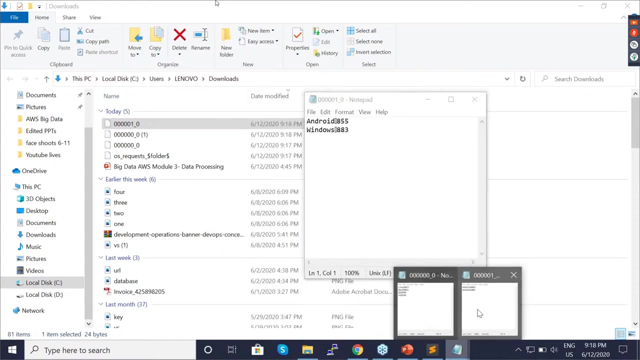 so, as i told you, the output would be, uh, the os name and the number of hits, and you can see this. let me open this as well. yeah, okay, i think you're able to see. right now we can see: android: 855 hits. windows: 883 hits. 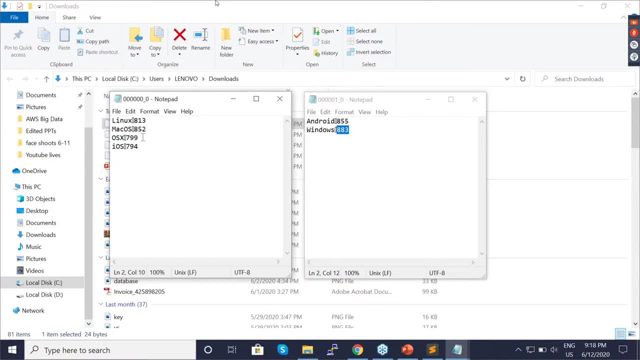 linux 813, mac 852, osx, which is for the apple laptops, uh, macbooks, so it's 799 and in ios it's 794. so we've got the files, guys, over here. so this is this actually means that our program ran successfully. we created a hive, sorry, we created an emr cluster. successfully, we ran a. 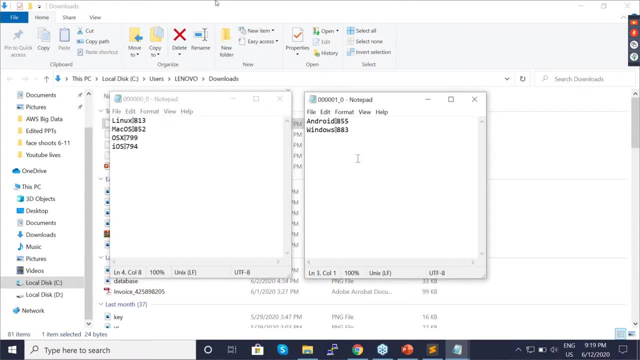 hive program on it and we also got an output. the thing is, this file is very small. that's why we got an output in less than a minute. but if your file is very, very large and it takes a lot of time to process, then obviously it will take around 10 to 15 minutes, according to the size of your 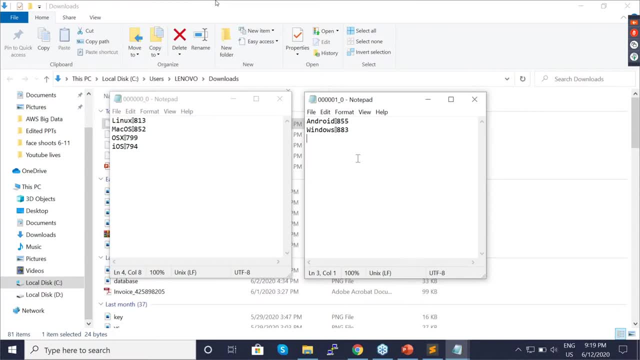 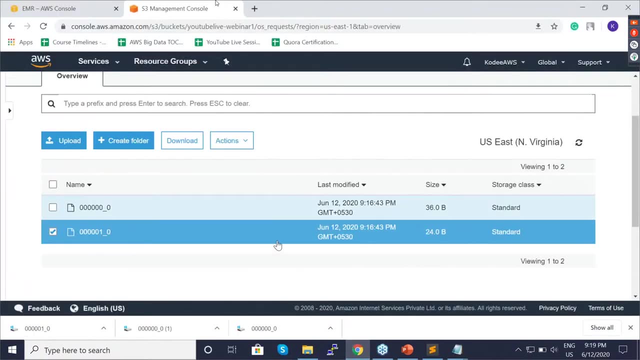 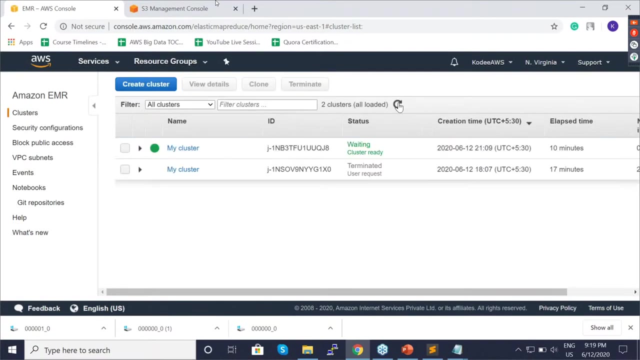 file, and sometimes it can also take a horse because you might have, let's say, petabytes of data. okay, so we've come to the end of this session. so, going back over here, we've successfully created the cluster. we ran a hive program, and both of the steps have succeeded. 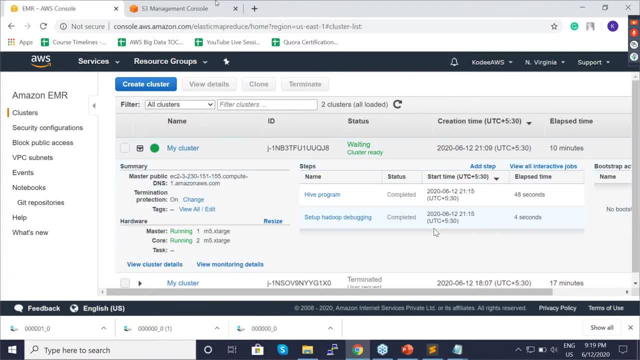 you can just click here. yeah, so both of the steps have been come, uh, succeeded. so it is waiting because right now there is no process running. if you want to add a process, you can click on step and add another program to run your program and process data. so 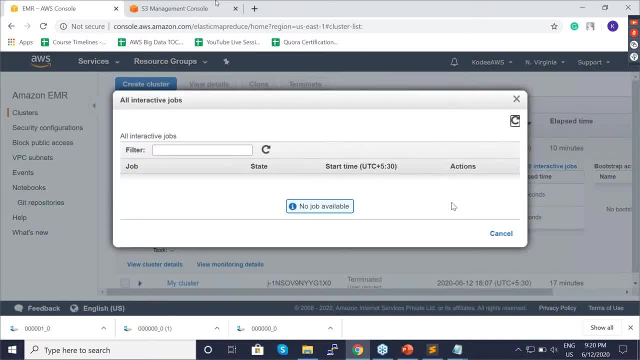 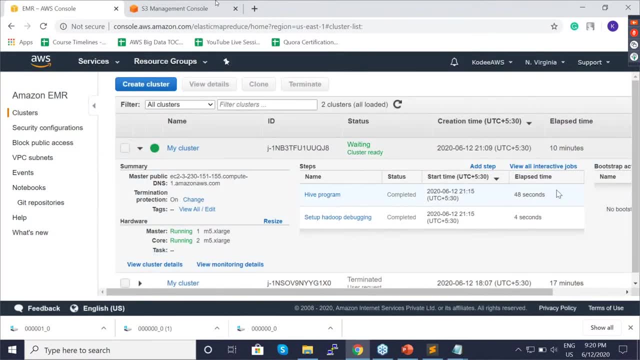 you can do that. you can see all the interactive jobs over here. if there is any current job running, you can see the job. so, for example, we were running this hive program, so while running we could have seen that job over here. so the thing is, this cluster can be shared. 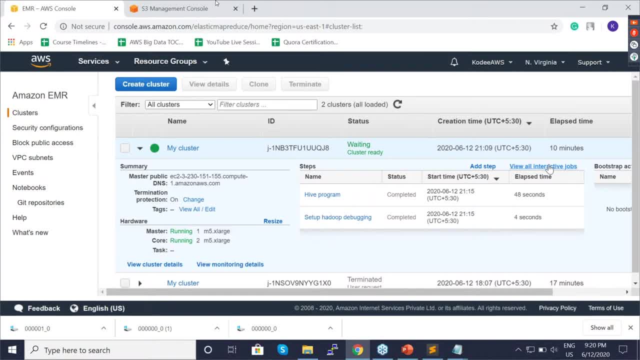 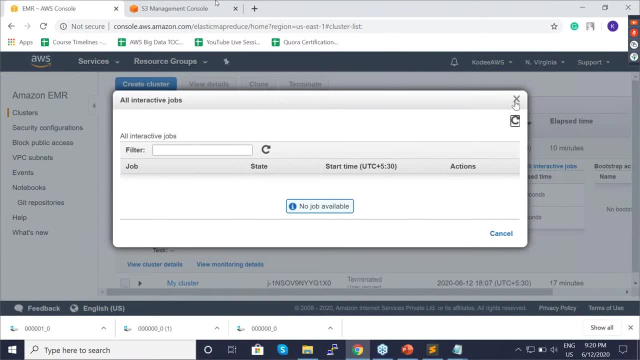 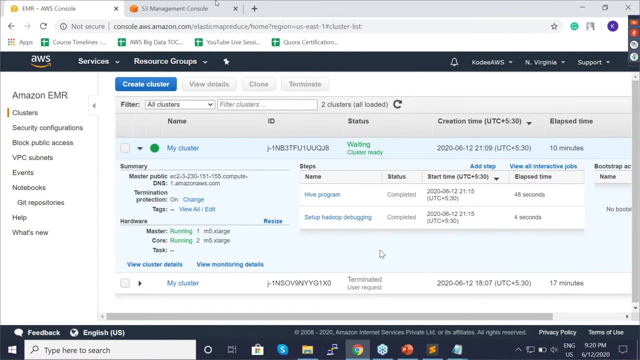 among other users in my aws account, so that all of them can run a job at the same time and we can check all the jobs running over here. so i think that's pretty much it. so it's pretty simple to start off with this. it's pretty simple to create a cluster. run your own program with your own input. 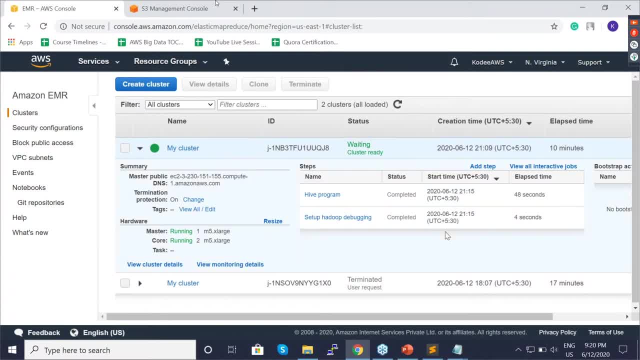 data set. the thing is, while running the hive program, we gave an input data link. so instead of providing that link, you could, you could provide your own data set, and then here we'll go to our set and you could provide your own hive script and you could provide your own output location.